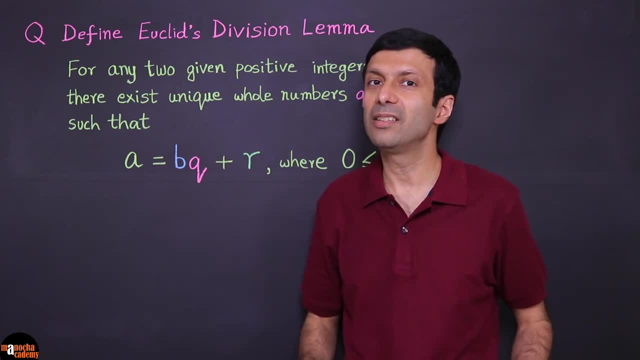 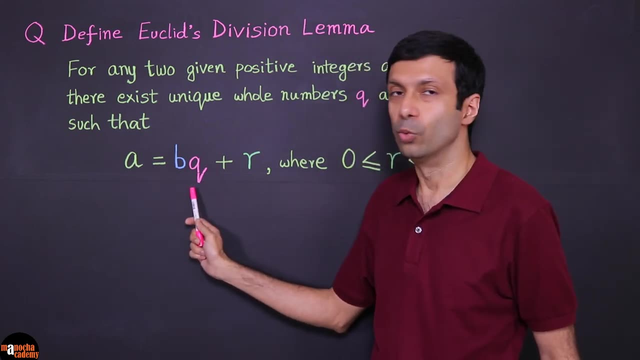 and you divide A by B, then you will get a quotient and a remainder right. So if you divide A by B, A is called the quotient Q and the remainder R. So what is A called? It's called the dividend right. 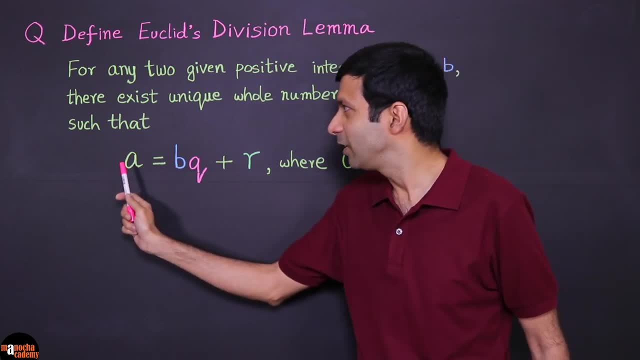 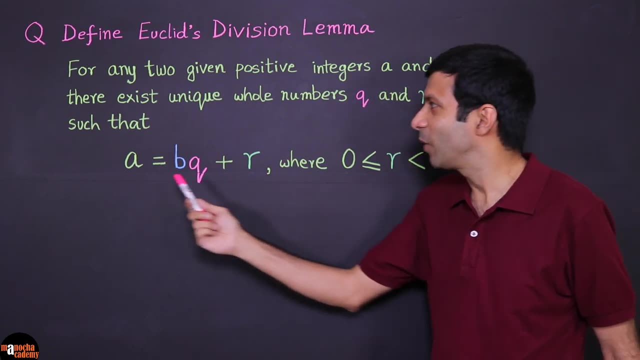 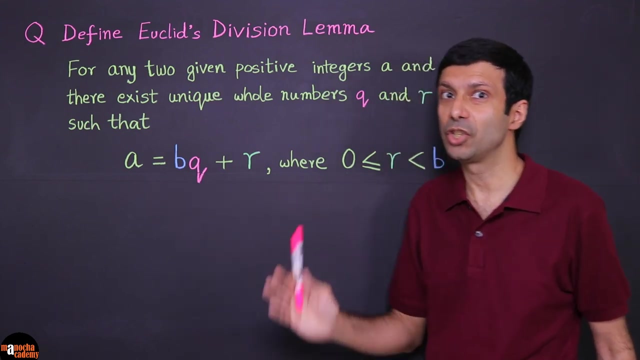 And B is our divisor. So when we divide the dividend A by the divisor B, the quotient is Q and the remainder is R. That's why we can express it in this form: A equals BQ plus R. Now what is the condition on the remainder R? 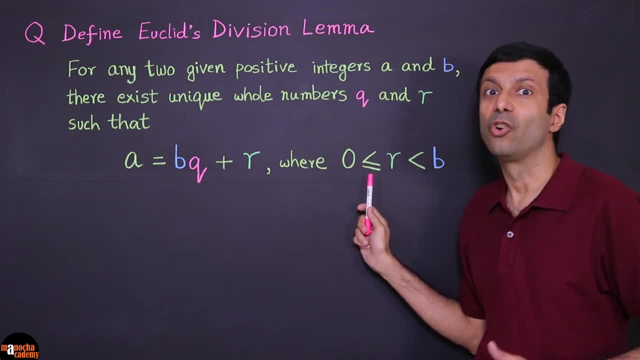 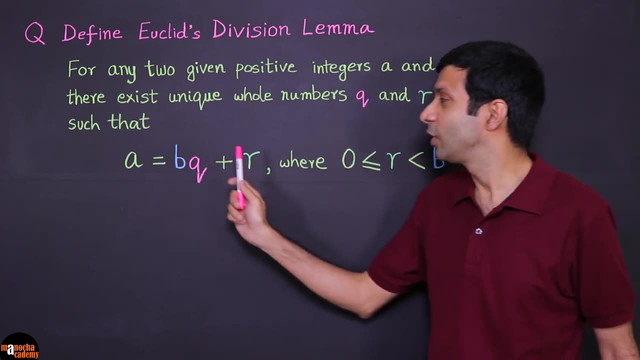 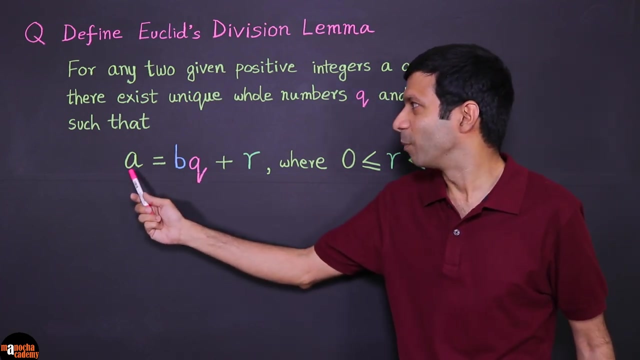 You know that the remainder R will obviously be greater than 0. And it will also be less than B. Why? Because you are dividing by B, So the remainder can't be greater than B. So we can express it in this form: 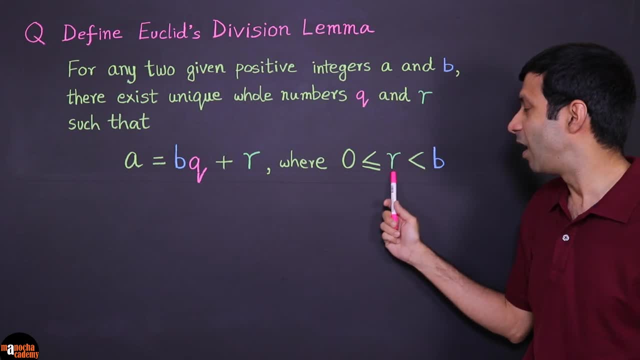 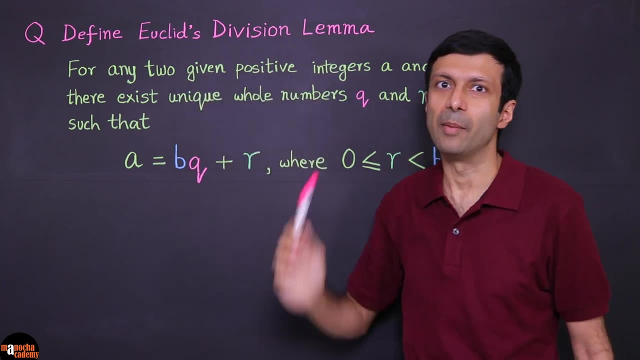 A equal to BQ plus R, where- remember R- the remainder is greater than or equal to 0 and less than B. That's Euclid's division lemma. Now let's look at this question Using Euclid's division lemma. 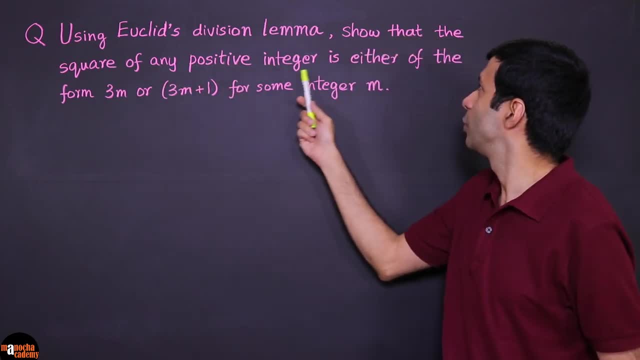 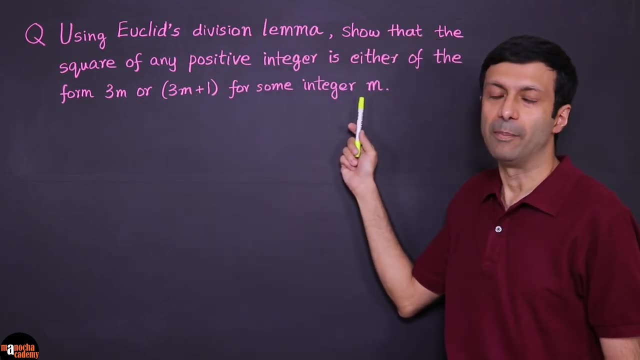 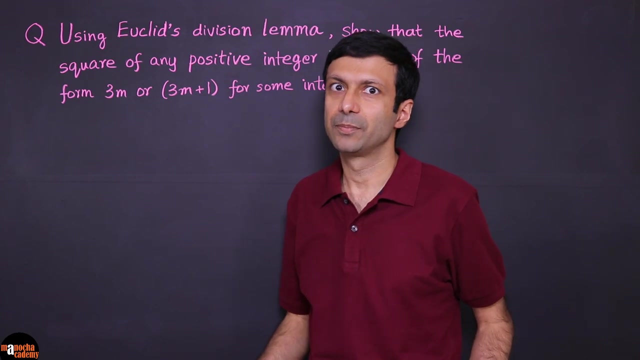 show that the square of any positive integer is either of the form 3M or 3M plus 1, for some integer M. Okay. So let's take any positive integer, Let's write it as N. And now, if you take N, 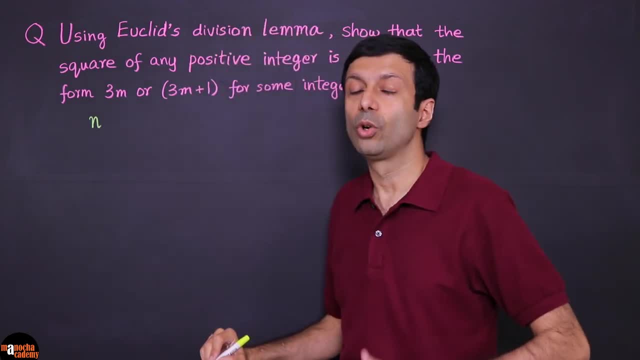 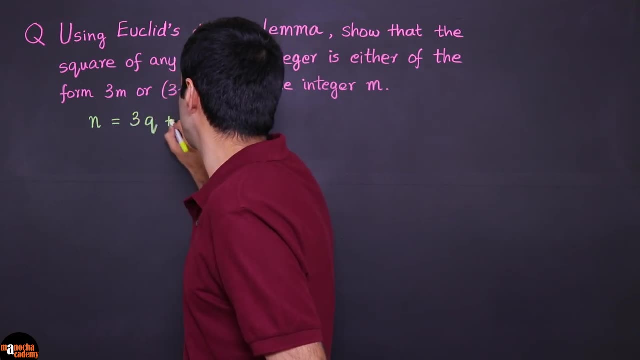 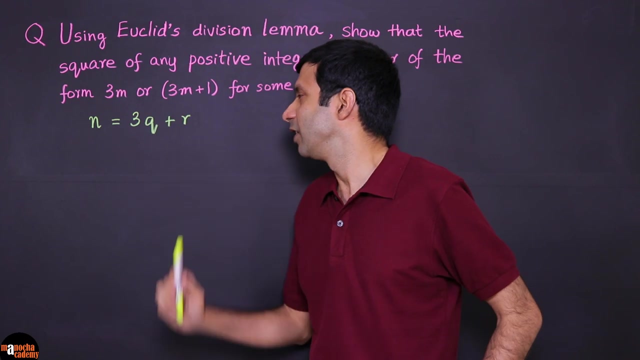 and if you divide it by 3, then, using Euclid's division lemma, we can write it as N equals N equals 3Q plus R. Right, Because, remember, Q is the quotient and R is our remainder here. So what is the condition on R? 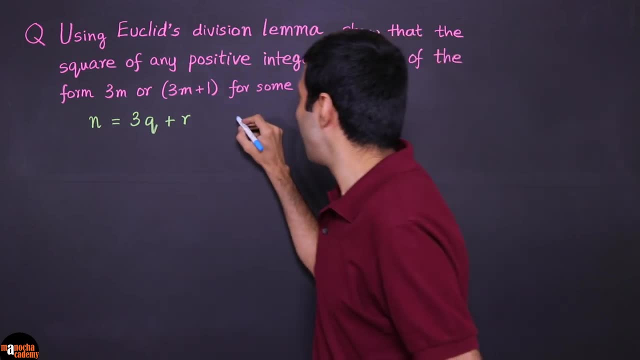 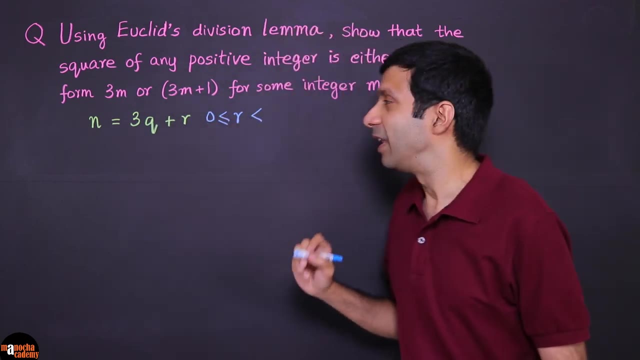 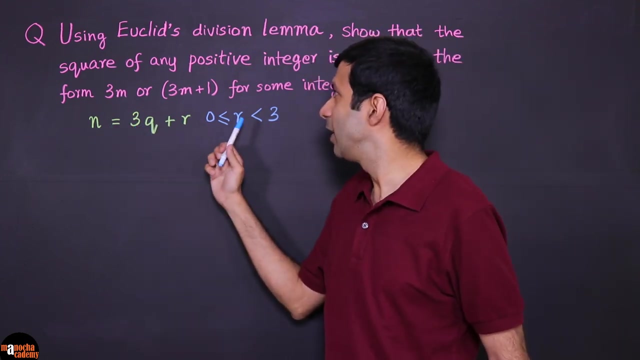 That's right. Remember: R is going to be greater than or equal to 0 and R is going to be less than 3.. Why? Because we are dividing N by the number 3.. So the remainder is either going to be greater than 0. 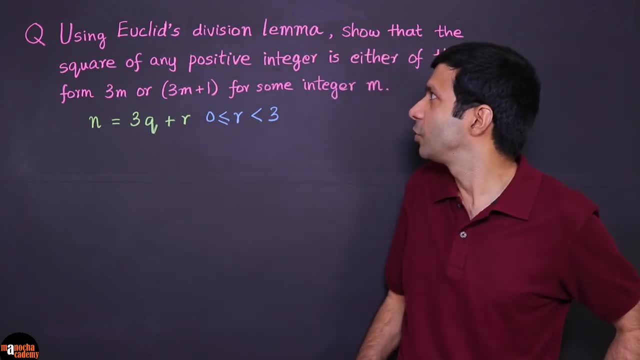 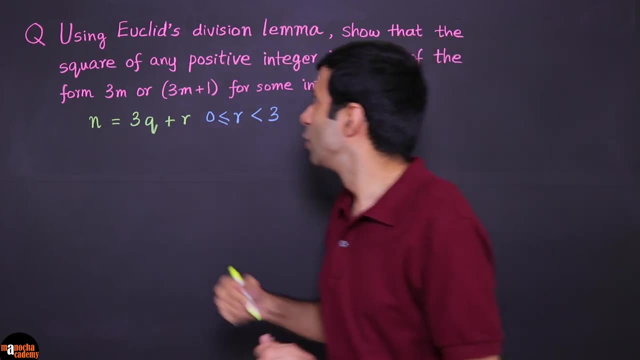 or less than 3.. Now, what does the question say? The question asks us to take the square of the positive integer. N was our positive integer right, So let's take its square. So what is N square going to be? 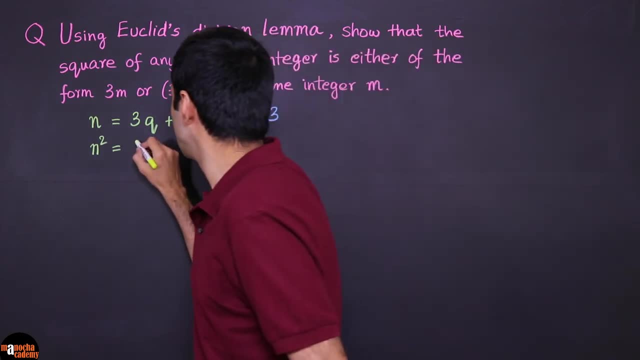 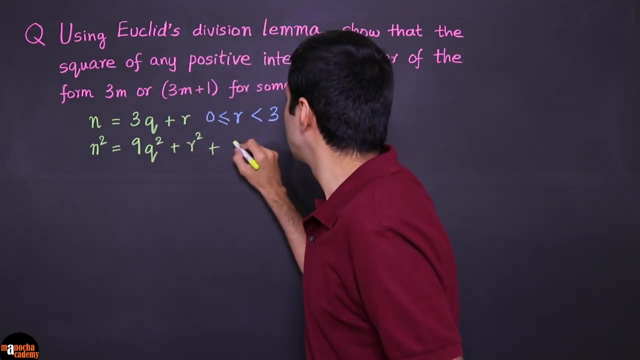 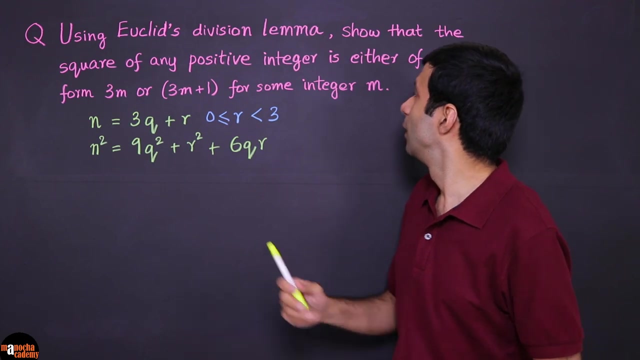 So simple. just apply the A plus B whole square formula. So we are going to get 9Q square plus R square plus 6QR, Right? So that's the N square, And now we need to show that N square, the square of this integer. 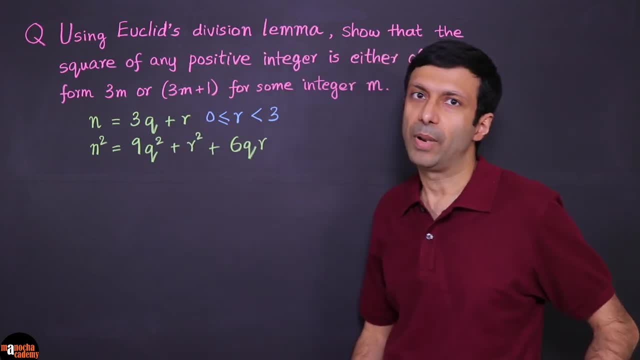 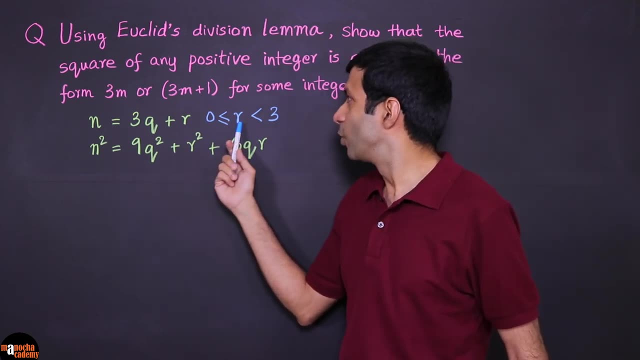 is either of the form 3M or 3M plus 1.. Okay, So for that we need to consider three cases, right, Because either R can be. So what are the possibilities of R, Since it's between 0 and 3,? 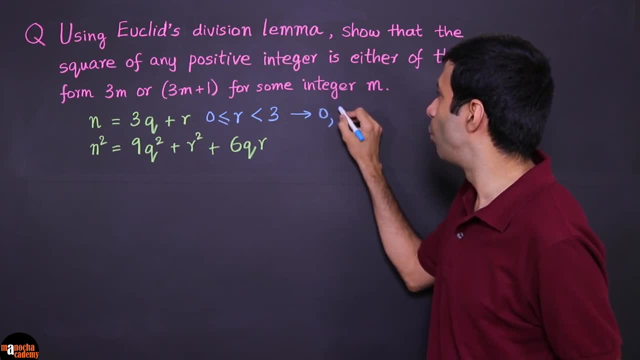 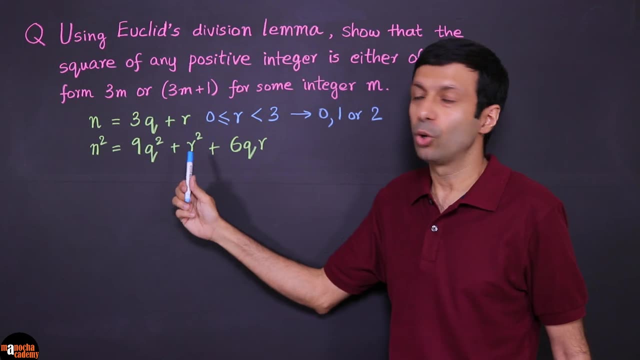 R can either be 0,, 1, or it could be 2.. So that's why we need to consider these three cases and show that the square is of this form: either 3M or 3M plus 1.. 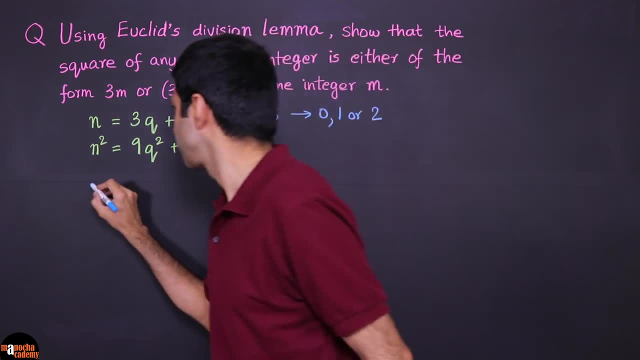 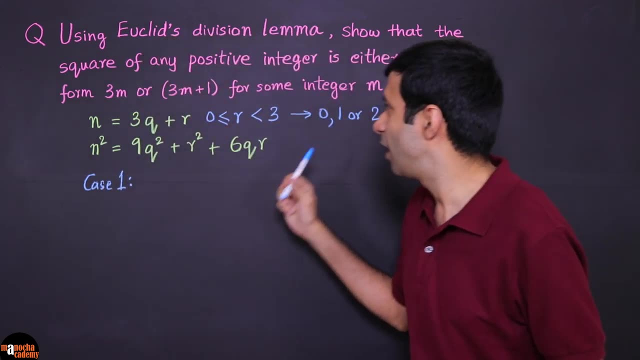 Okay, So let's start with our first case. So our case 1 is going to be Right. What is our case 1?? R equal to 0.. So let's substitute R equal to 0.. So let's substitute R equal to 0. 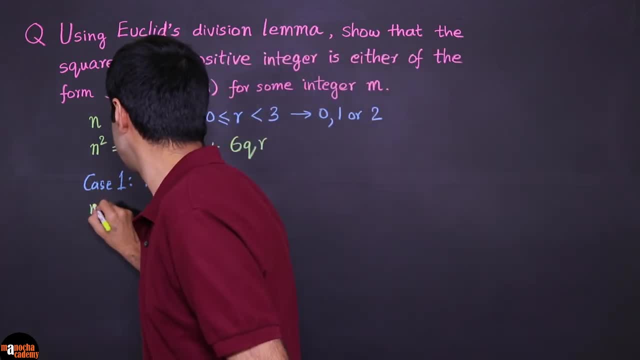 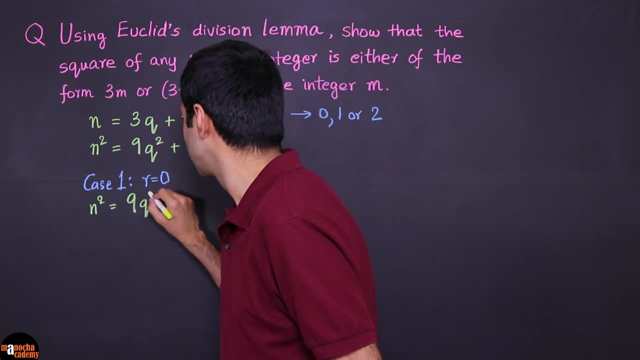 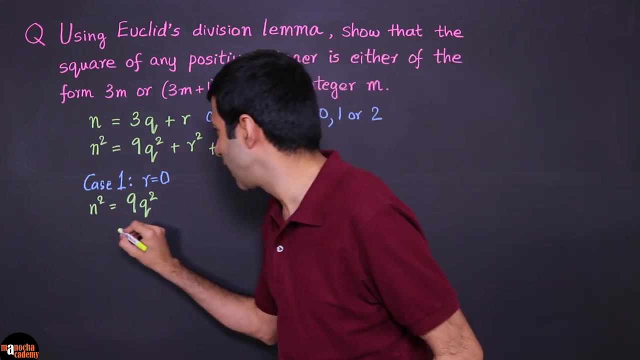 in this square, And what are we going to get? N square is going to be 9Q square And R is 0.. So these terms go away, Right. So now let's We can write this as 3. 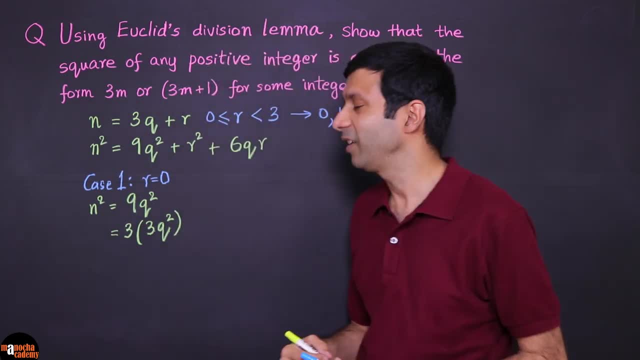 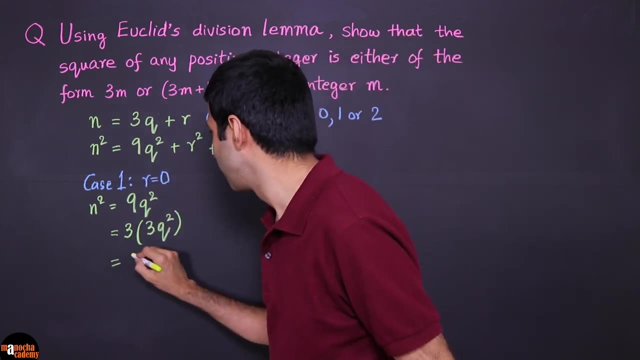 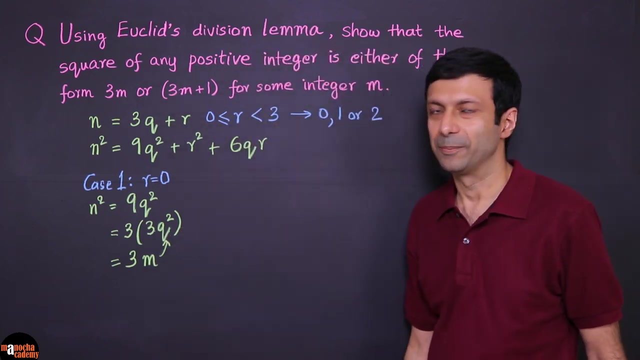 into 3Q square. Okay, Right, And so here you can see: if we take 3Q square as M, this is going to be of the form 3M, where M is basically your 3Q square, Okay. 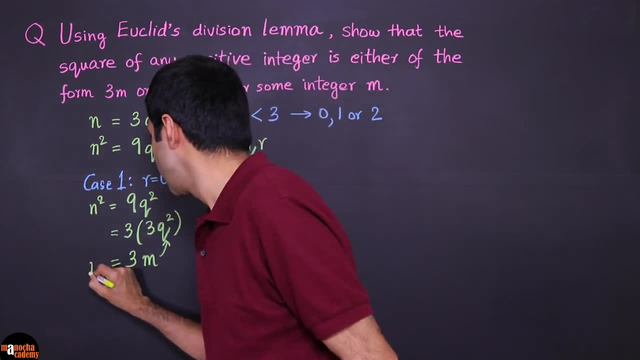 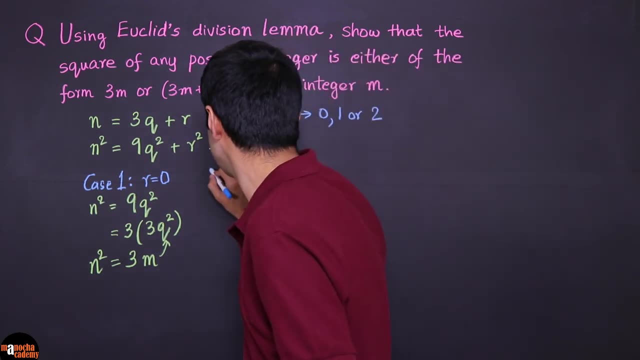 So this is our case 1.. So we've shown that N square is of this form: 3M. Now let's look at our next case, case 2.. So case 2 is going to be what? 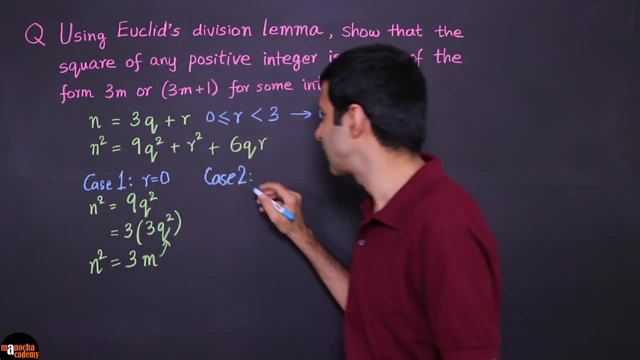 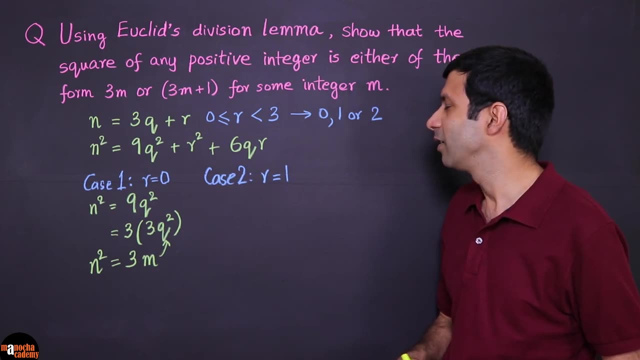 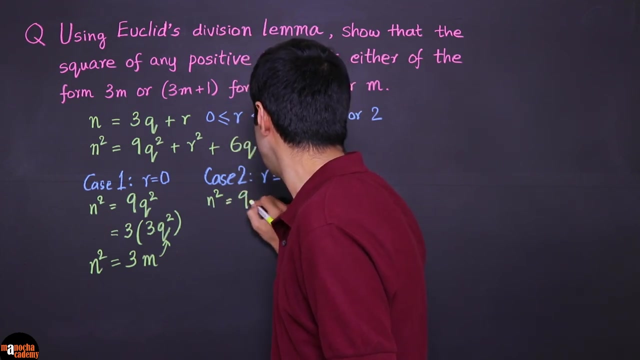 Where you need to take R equal to 1.. The next case: Okay. So again, pretty simple. We're going to substitute the value of R in N square. So what are we going to get here? N square equals 9Q square. 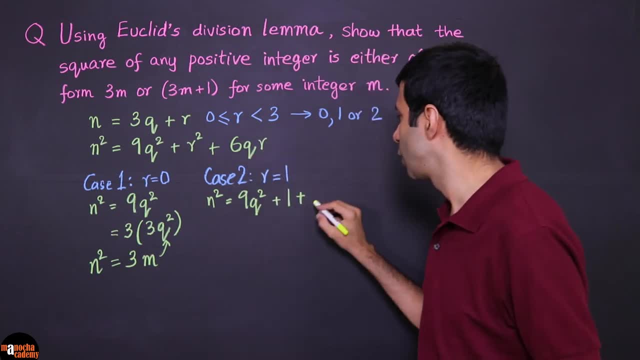 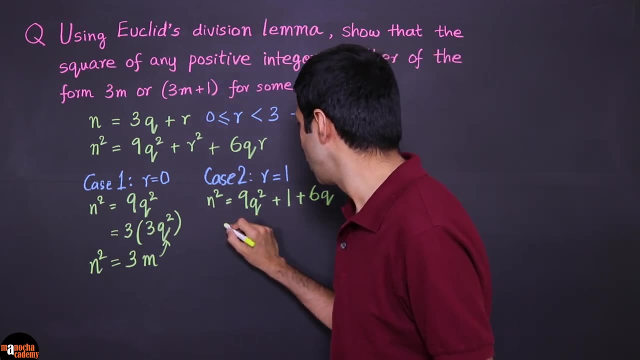 R square, So that's 1 plus 6QR, 6Q, Right, So we've substituted R as 1.. Okay, And so now let's rearrange this a bit. We can write here as 9Q square. 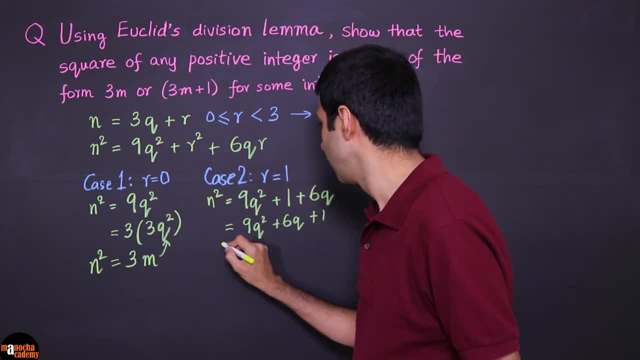 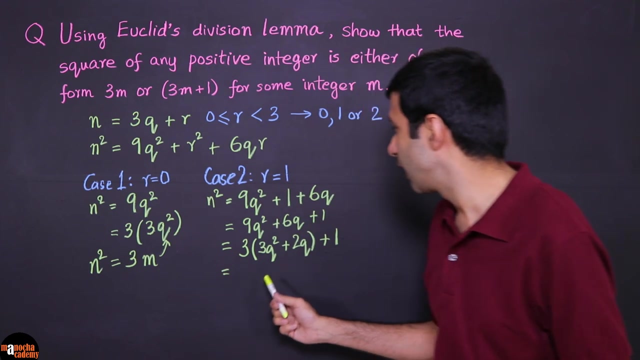 plus 6Q plus 1.. And let's go ahead and take 3 in common here. So it's going to be 3, 3Q square plus 2Q Plus 1.. Right, And so can you see again. 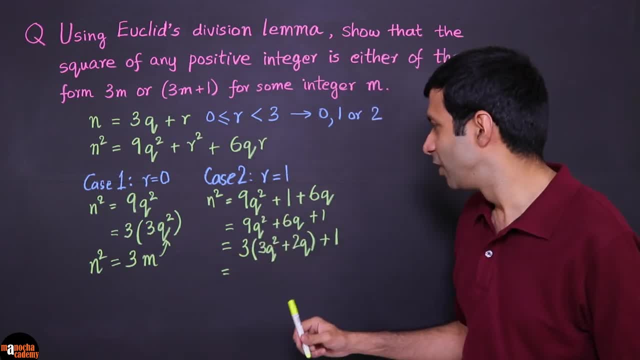 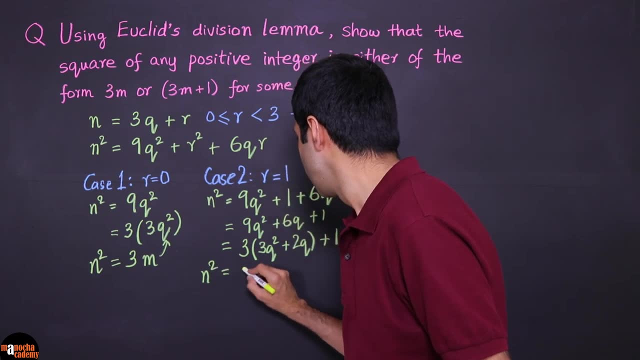 if we take this 3Q square plus 2Q as an M, so M where M is any integer right, Some integer, So N square becomes of the form 3M plus 1. Right, So it's matching. 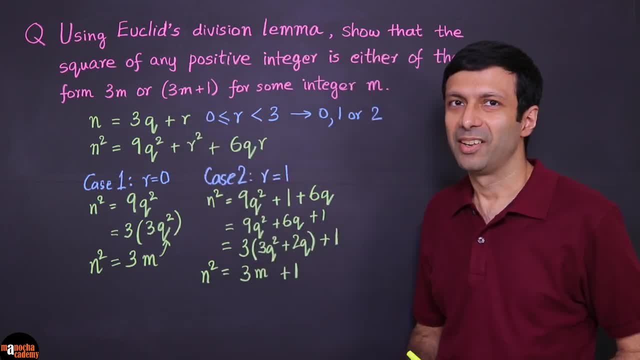 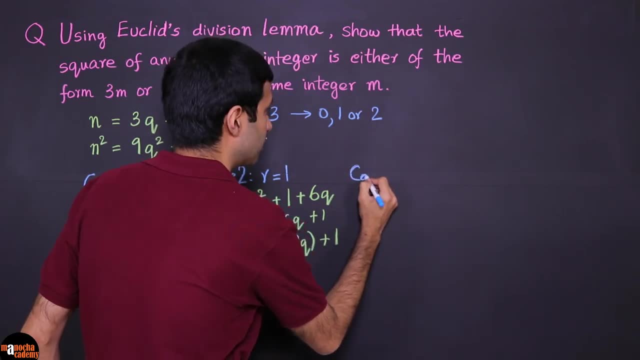 So in this case 2, it's of this form- 3M plus 1. Right, Simple. Now all we have left is with our last case, Case 3.. And what is case 3 going to be? 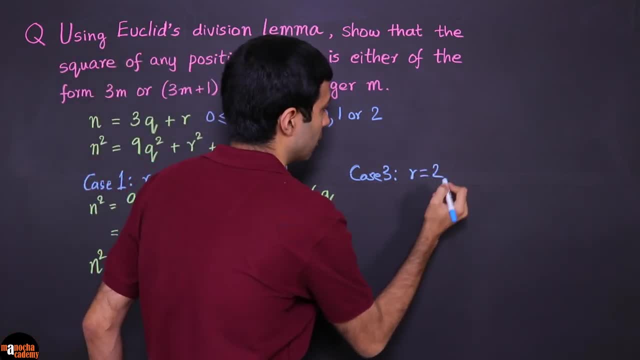 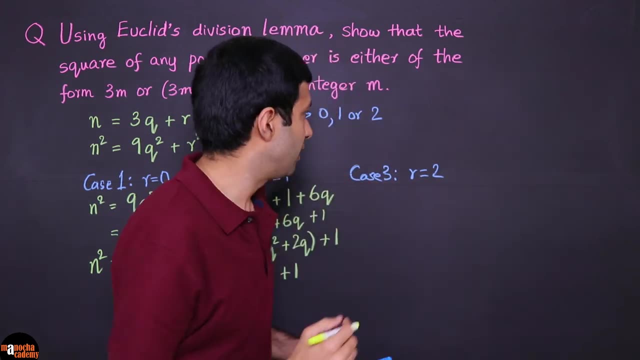 We're going to take simple R equal to 2.. Okay, So let's go ahead and substitute that in this form, right? The N square. So let's write it as N square is going to be. So go ahead and work with me, right. 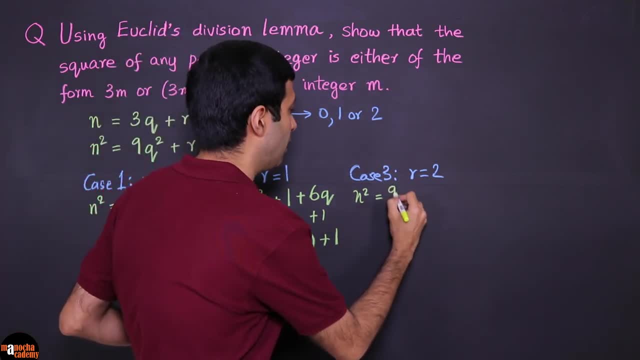 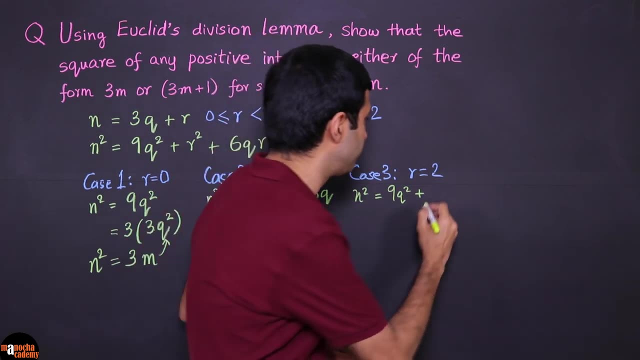 You can also try this yourself. It's pretty simple. So it's going to be 9Q square plus we have R square, So that's 4.. And we have plus 6QR, So what is that going to be? 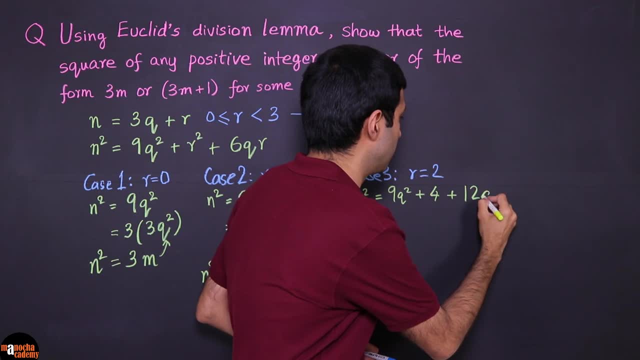 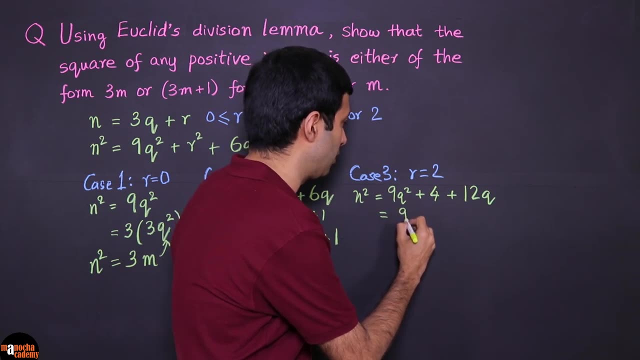 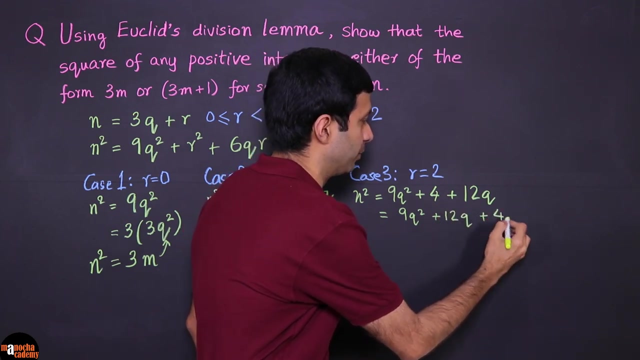 12Q. Pretty simple. Now let's go ahead and write this as 9Q square plus 12Q plus 4.. And now again, we need to either have it in the form of 3M or 3M plus 1.. 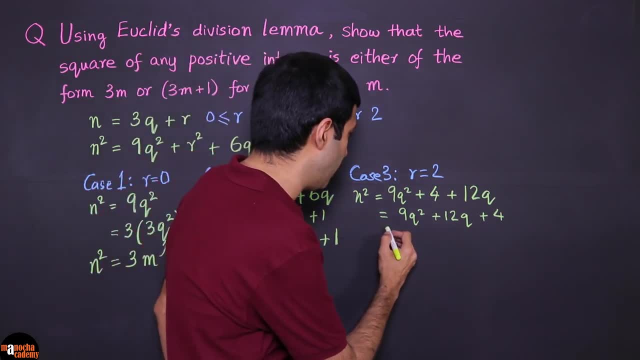 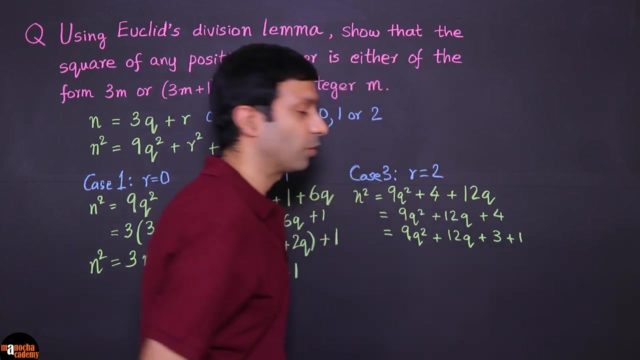 So let's see what do we get here If we break this down as 9. sorry, this is 9 Q square plus 12Q plus 3 plus 1.. Okay, So I'm just going to split 4 into 3 plus 1.. 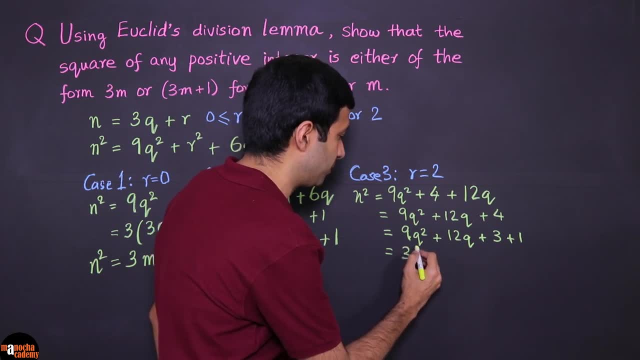 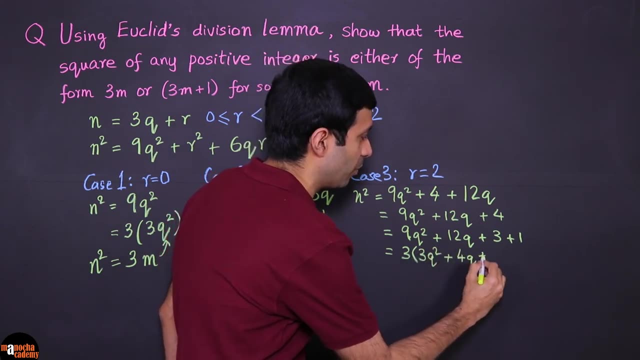 And now, if we take 3 common here, So we are going to get 3 into 3Q square Plus 4Q plus 1 plus 1.. Right, And can you see our form? 3M plus 1, right here. 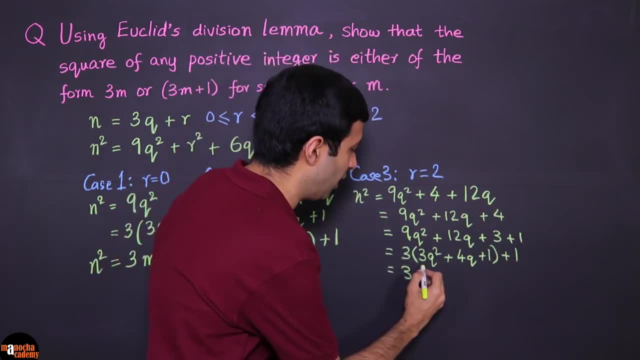 It's very simple: Just take the 3 and this whole thing is in. So this whole thing is going to be our M here, M Okay, which is basically 3M plus 1.. So this is our M here: 3Q square plus 4Q plus 1.. 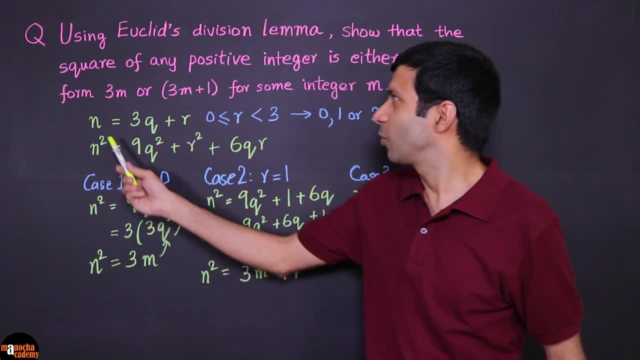 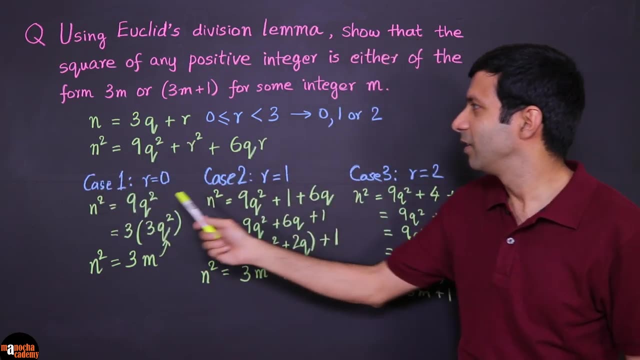 So see, we've solved our question. What did we start with? We took N, where N was divisible, divided by 3, and then we took it square and we considered the 3 cases And in all the 3 cases we've seen, we've either got the form 3M. 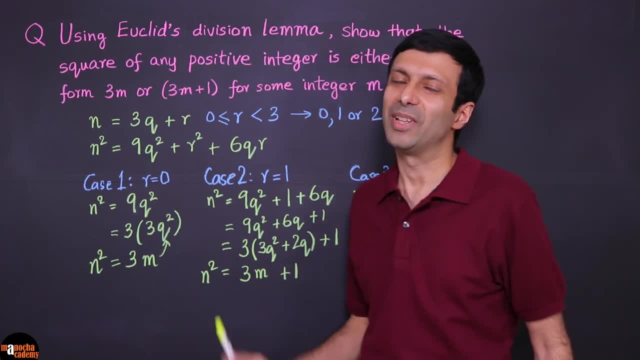 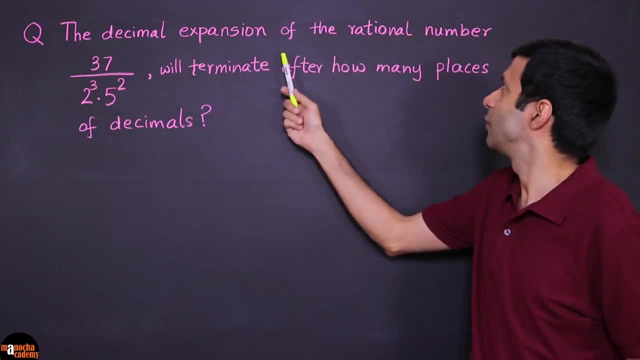 or 3M plus 1.. Right, So that's our answer here. Now let's take a look at this question. The decimal expansion of the rational number 37 by 2Q into 5 square will terminate after how many places? 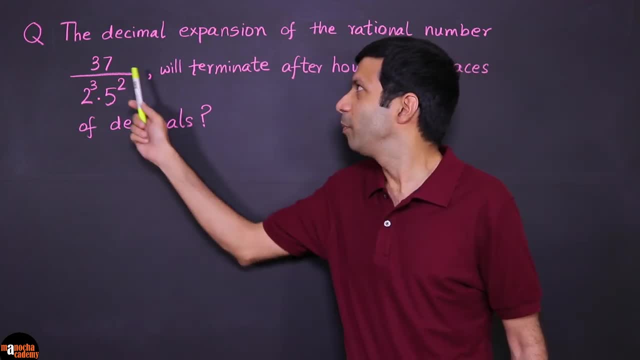 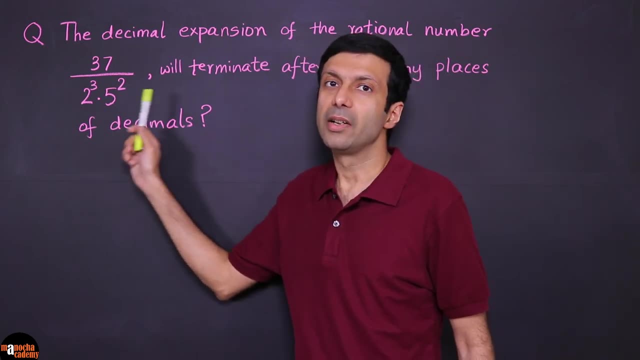 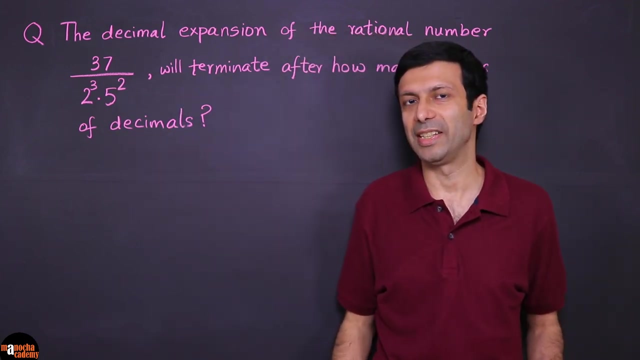 of decimals. Okay, So we've been given this rational number here. Now the first thing to check is whether this rational number will terminate or not. So if we write it in its decimal form, will it be a terminating decimal or a non-terminating decimal? 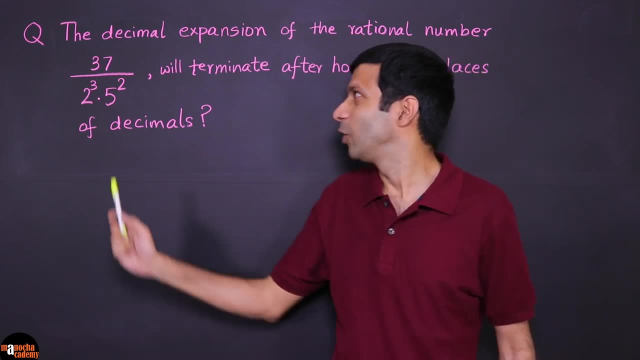 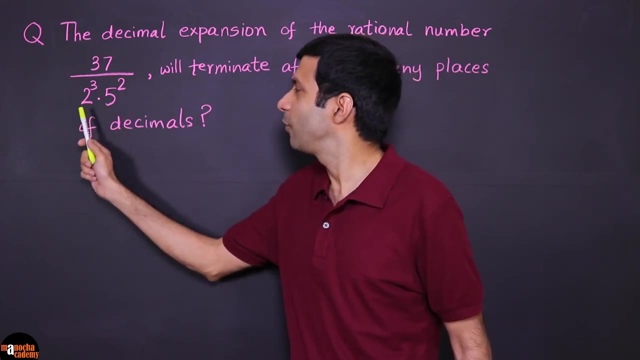 What do you think That's right? It will be a terminating decimal. Why? Because, as you can see, the denominator has only factors of 2 and 5. There's a 2Q and a 5 square, So only factors of. 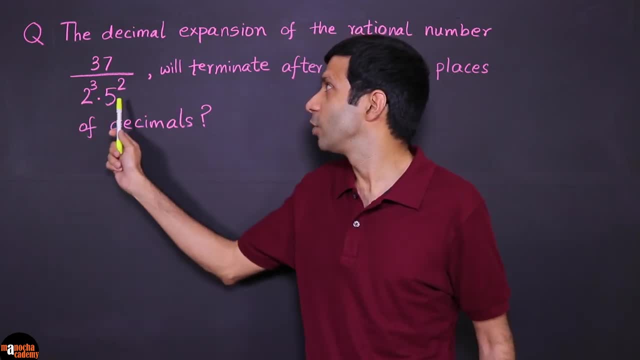 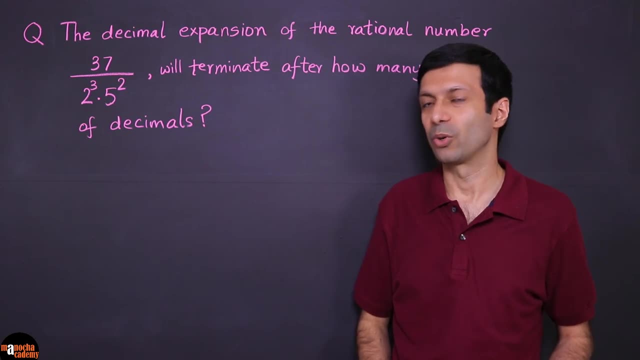 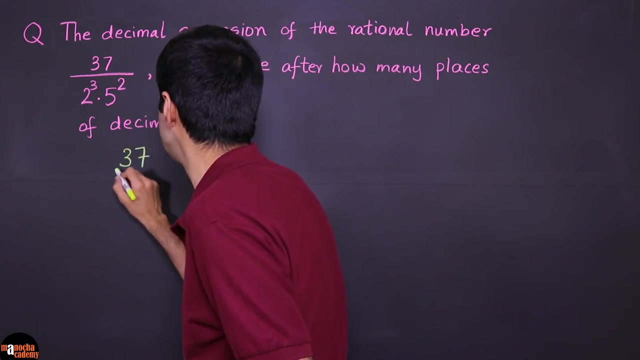 2 and 5. Nothing else. But if there was a into 7 here, Right, Then it would have been a non-terminating decimal. Okay, So let's write down our rational number. So we've been given 37. 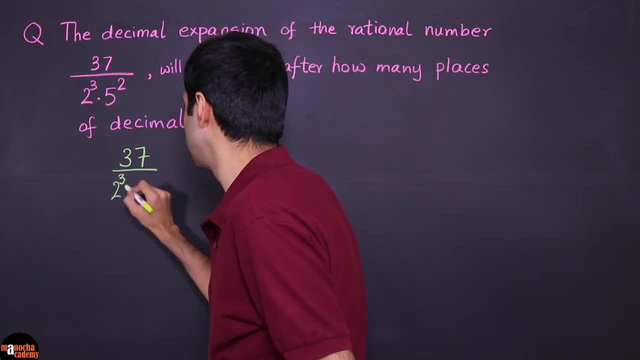 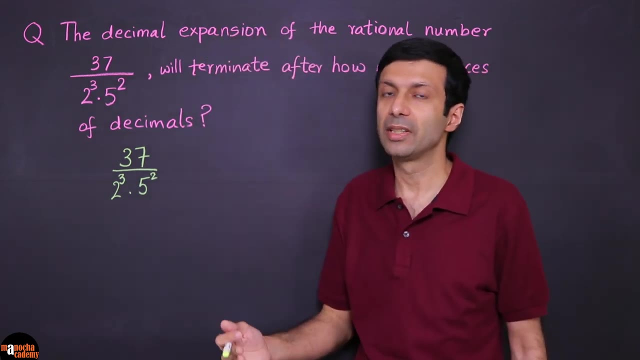 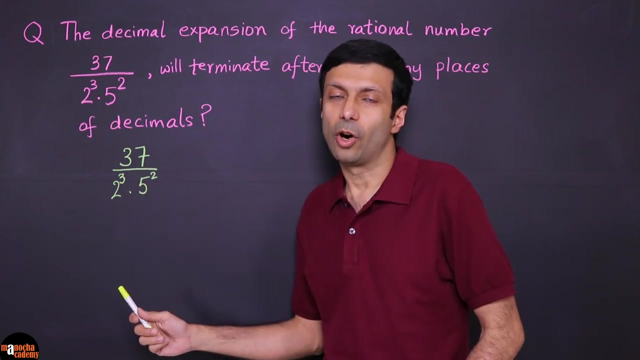 by 2Q into 5 square Right, And we need to find out after how many places of decimals will this guy terminate. So how do we solve that? So it's always convenient to turn the denominator into factors of 10.. 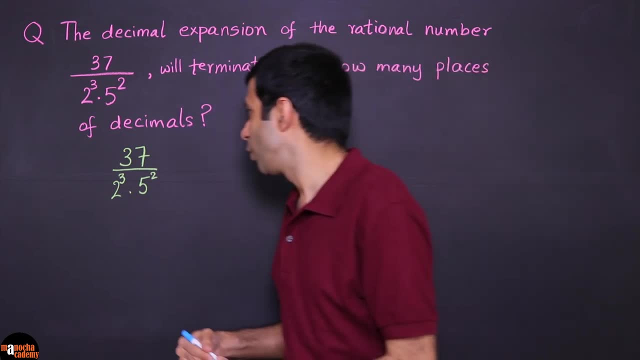 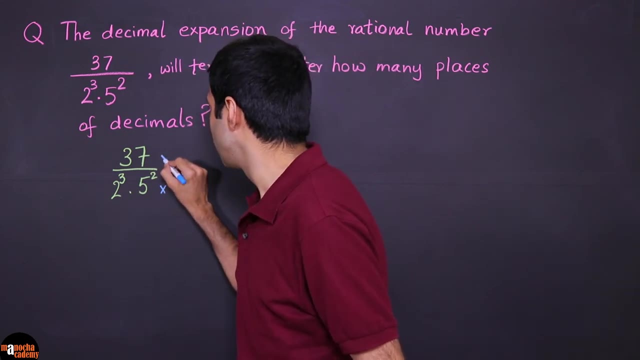 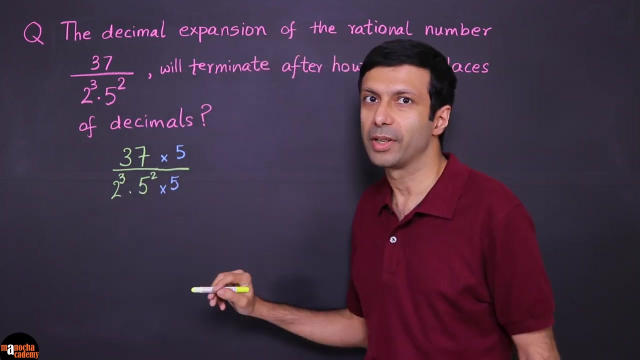 Right Into multiples of 10.. So here what we can do is multiply the denominator by 5.. Okay, And also the numerator by 5.. Why? Because we want. since we have a 2Q, we also want a 5Q. 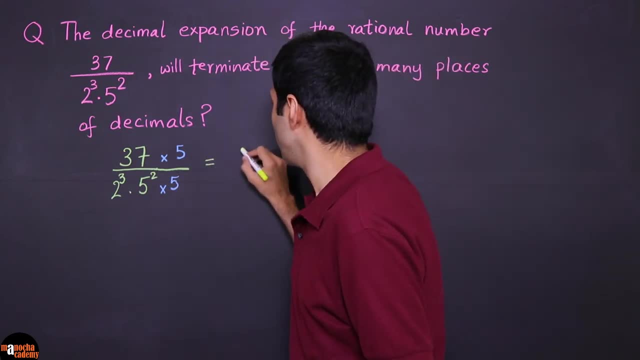 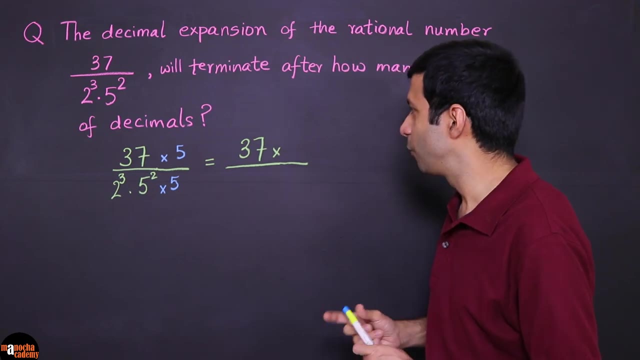 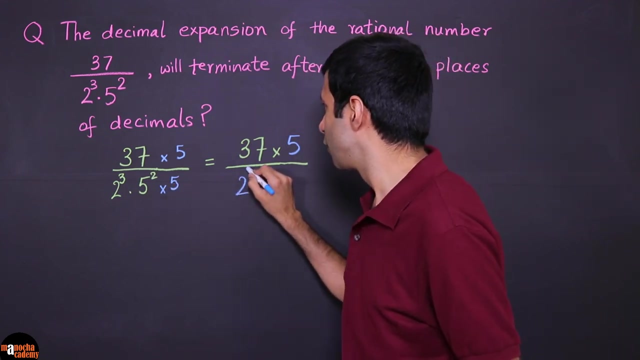 Right. So what does this become? So we are going to get 37 into 5.. So let me write the 5 in blue color here And the denominator is going to be 2Q into 5Q, Right? 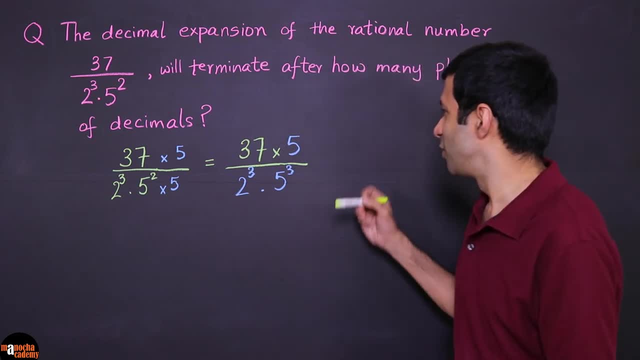 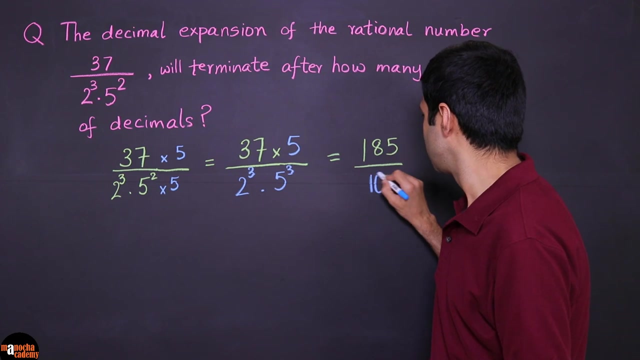 Okay. So what does this become? So, as you can see, so 37 into 5, we are going to get 185 here and divide it by so we will have a 10Q here, Right, 2Q into. 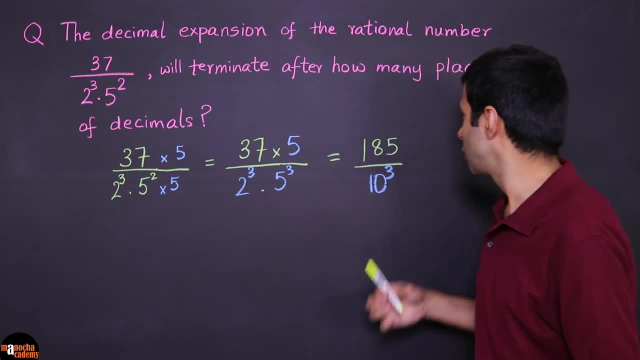 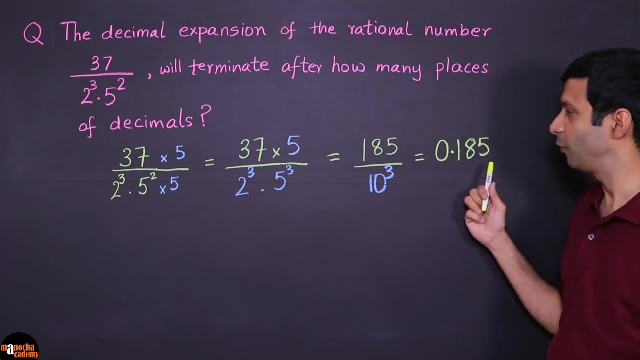 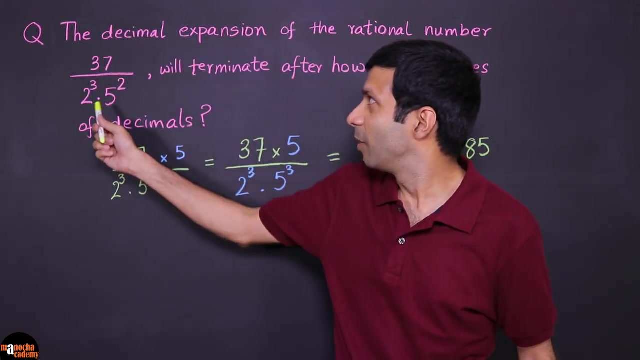 5Q. Okay, So you can solve this one and it's going to be 0.. 0.185. Right? So after how many places of decimal does this guy terminate? So the rational number that we were given. 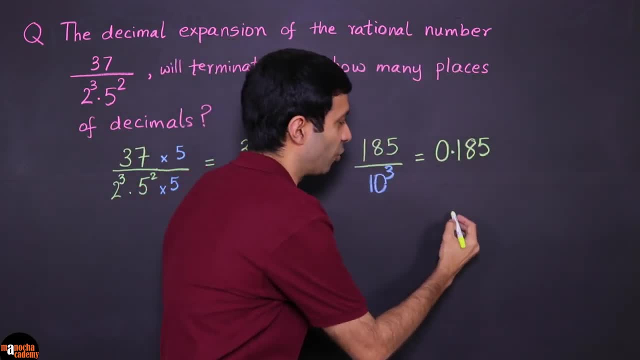 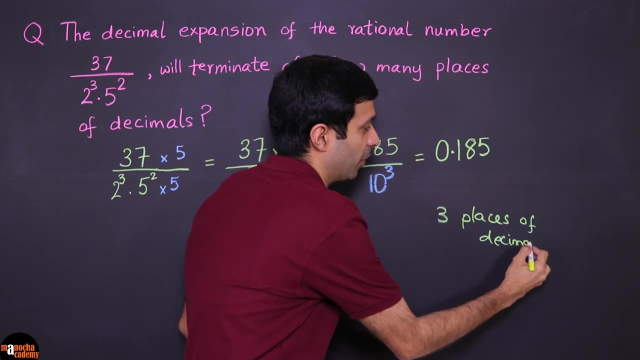 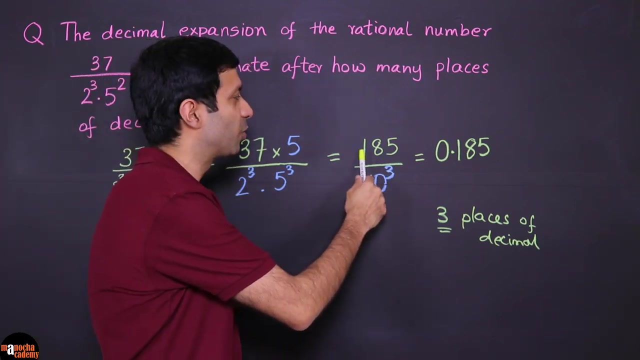 as you can see, it terminates after 3 places of decimal. So it terminates after 3 places of decimal. That's our answer, But we can also get it directly from here, because we know that it's 185 by 10 to the power 3.. 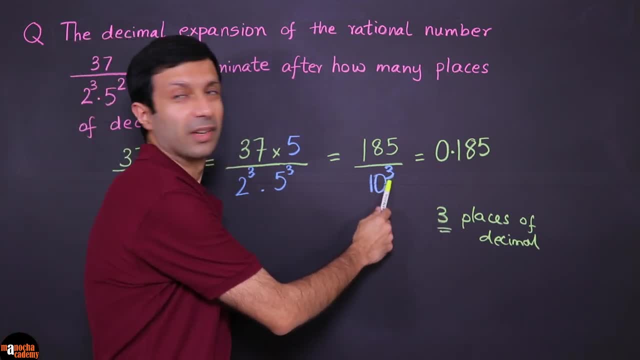 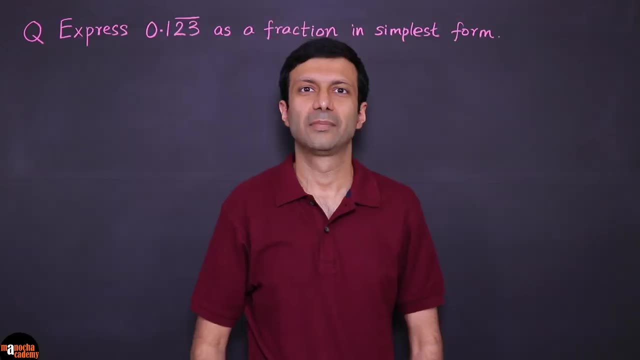 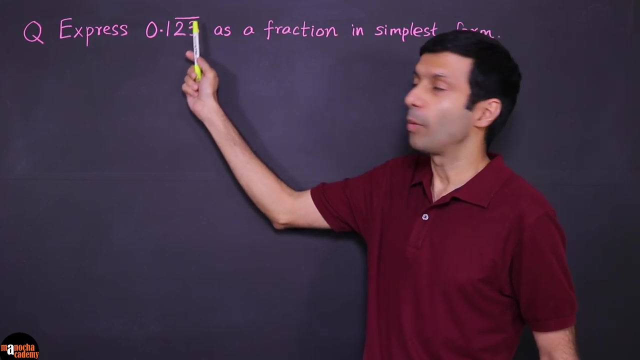 So we know that it will terminate after 3 places of decimal. Or if you solve it also 0.185, you can see that it terminates after 3 places. Let's take a look at this question: Express 0.123 with that bar on top of 2 and 3. 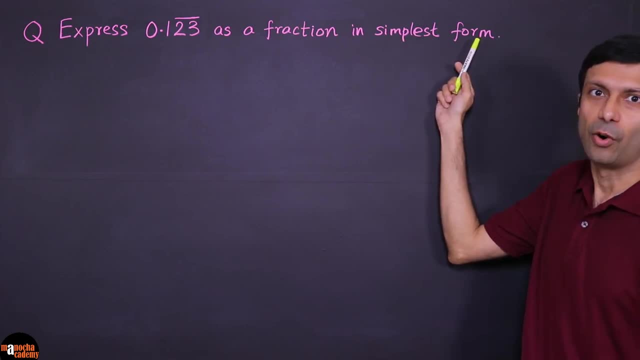 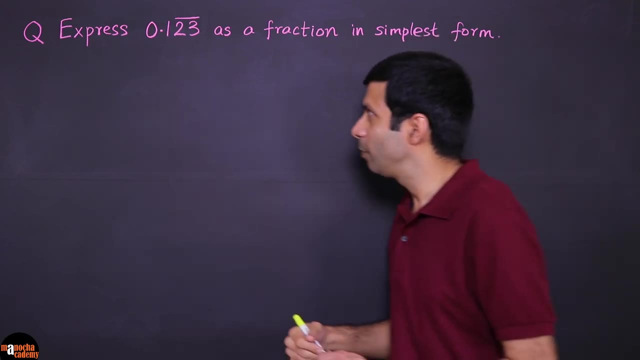 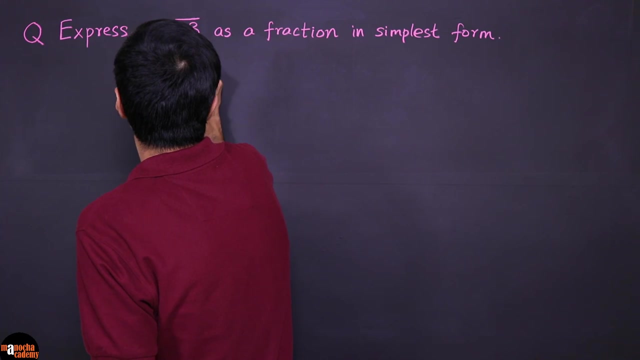 Right, As a fraction in simplest form. Okay. So how do you do this question? First, let's carefully look at this number. So what have we been given? 0.123 with that line, the bar on top, Okay. 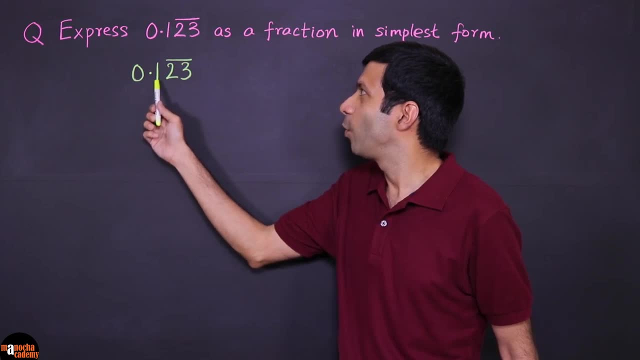 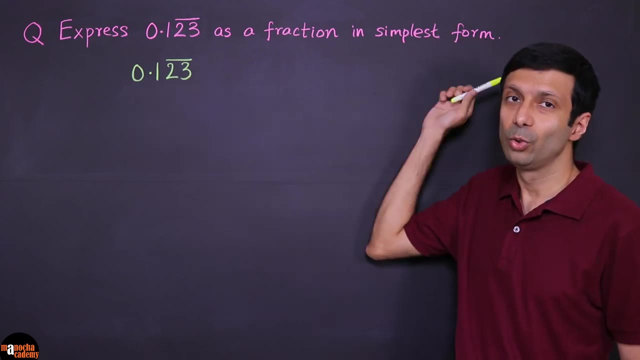 So what does that mean? This means that it is 0.1, with the 2 and 3 part is recurring, So it's like 0.123, 2 and 3, 2 and 3, 2 and 3. 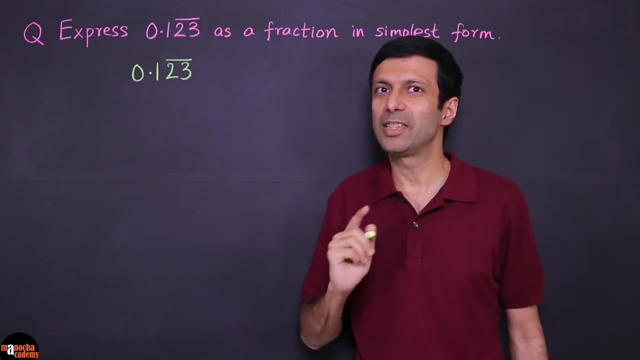 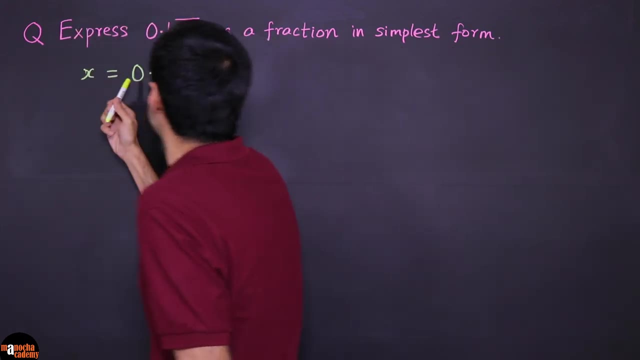 and it continues forever. So to solve these types of questions, what is the trick? You let the number to be x. So let's say the number x is 0.123, with 2 and 3 recurring Okay. So let's write it in a more expanded form as this: 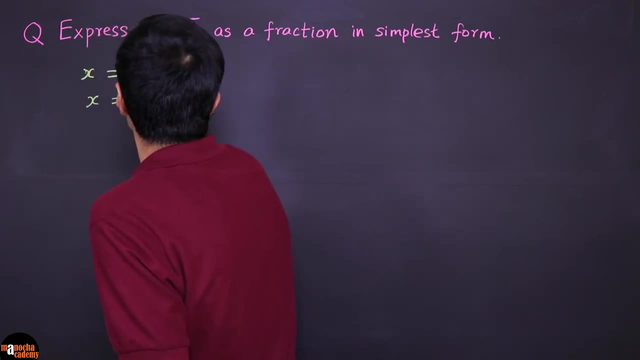 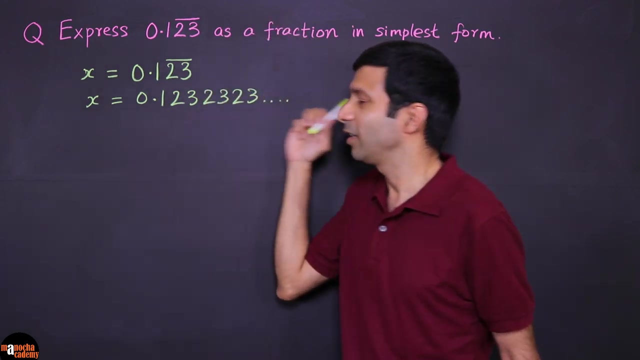 so that it's more clear. So x is basically 0.123, 2 and 3, 2 and 3 and so on. Right, So this keeps on repeating. Now we want to express this decimal number as a fraction. 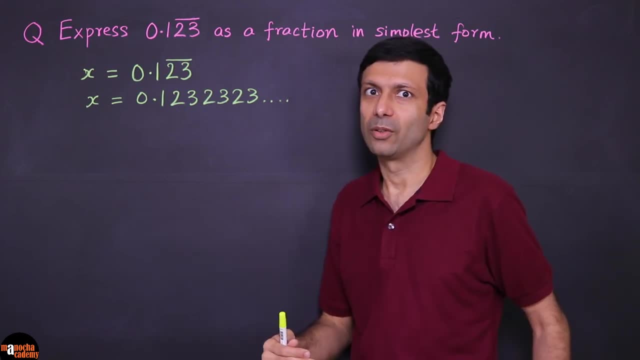 Right, Like in a p by q form. Okay, So typically, what's the trick? You try multiplying it by 10,, 100,, 1000.. Right, So let's first try writing. We will do it 10 times. 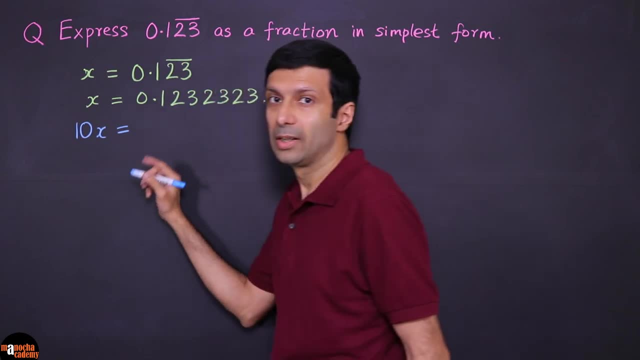 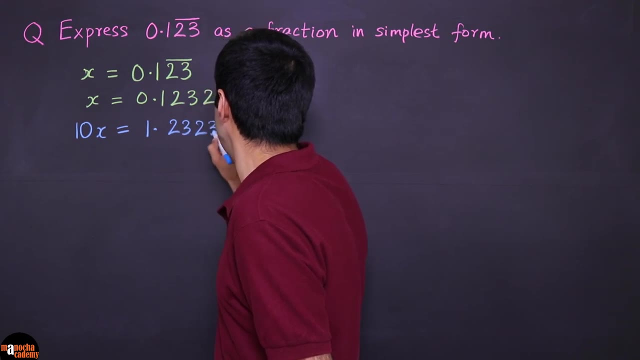 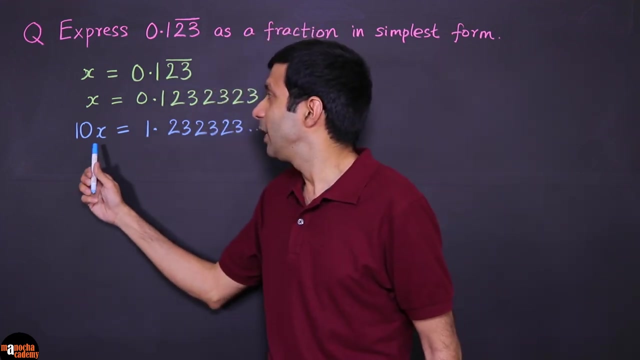 So 10x is going to be. So what will 10x be? Simply 1 point 2, 3, 2, 3, 2, 3 and so on. Okay, Now what we need to do is: 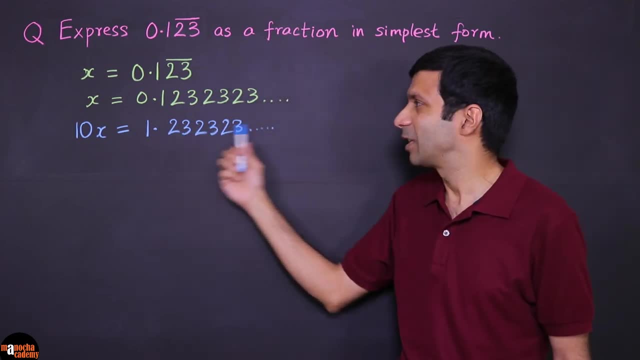 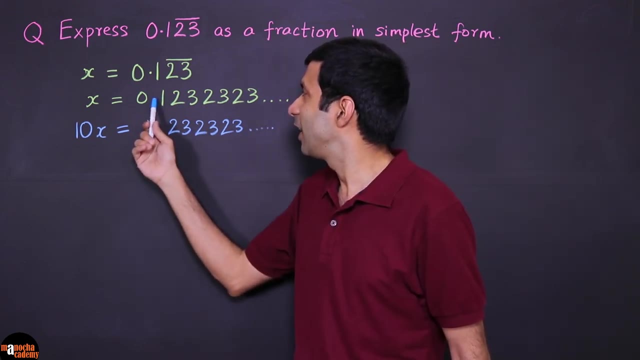 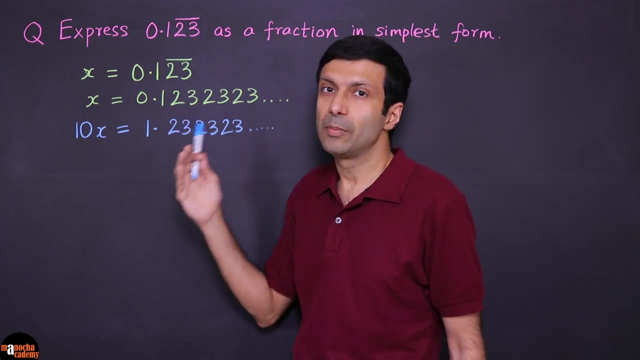 we need to get rid of this Recurring decimal part. Okay, But if you do 100x, what will you get? So 10x was this and 100x is going to be 12.323232.. Okay, So note that the decimal pattern. 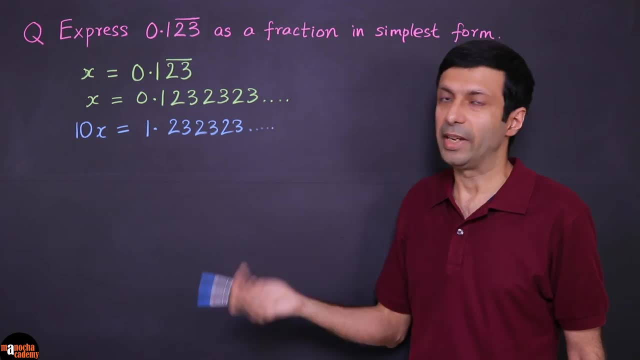 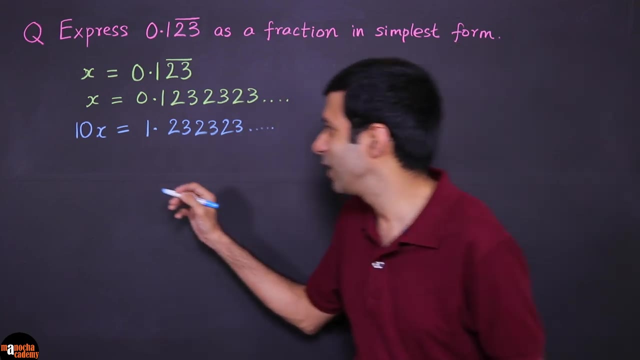 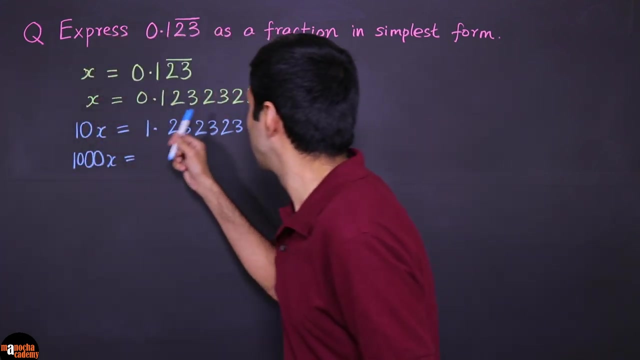 so the pattern after the decimal- sorry- will change if we do 100x, Right? So we don't want that. So let's try 1000x, Let's write down 1000x as, and that's going to be. 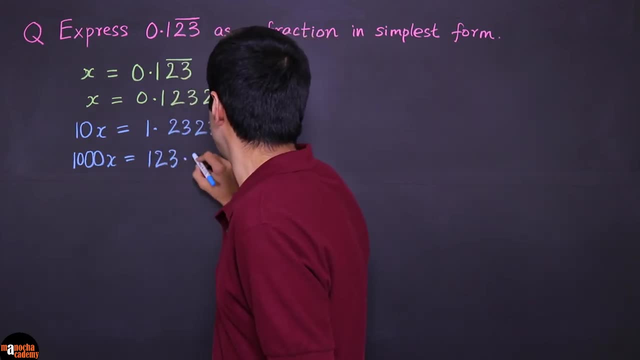 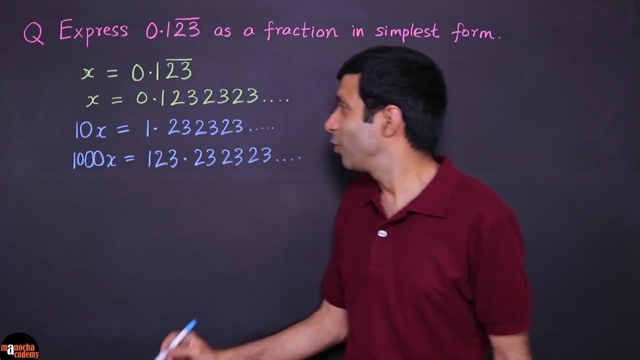 123.232323 and so on. Right, So now to get rid of this decimal part. Right, So the part after the decimal. it's pretty simple: We just need to subtract 10x from 1000x. So let me just copy down 10x here. 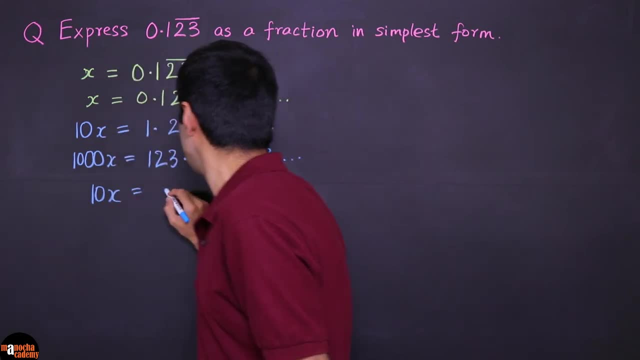 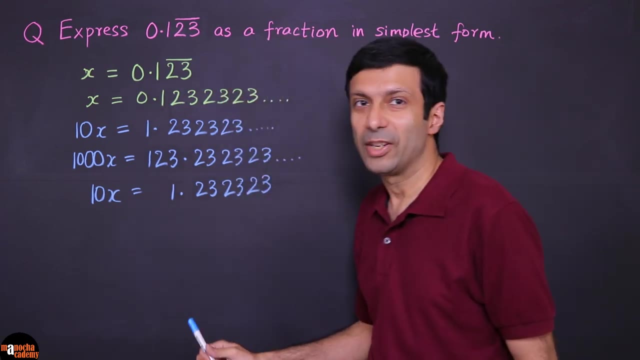 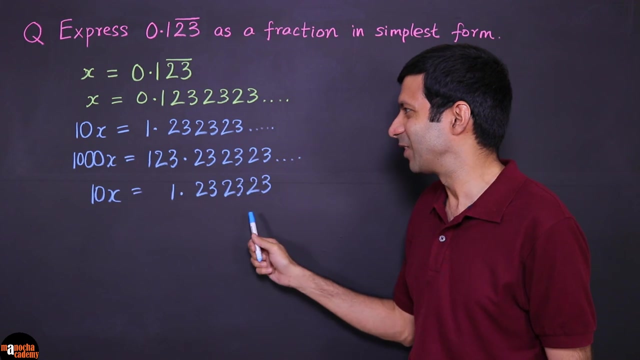 so that it's easy to see that. So let's write that down as So. can you see, If I subtract these two numbers, 1000x and 10x, this entire decimal part is going to get cancelled, Right. So let's go ahead and do that. 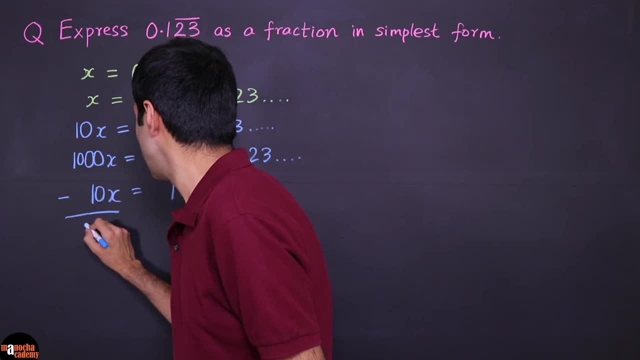 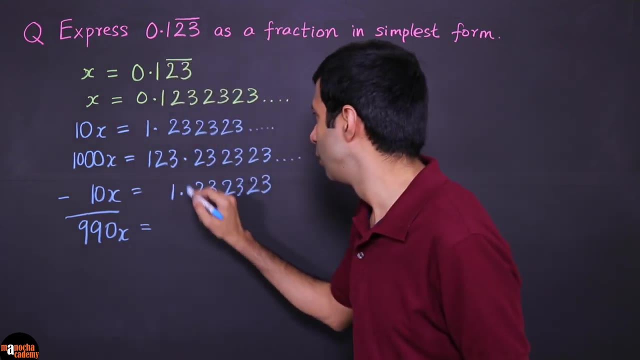 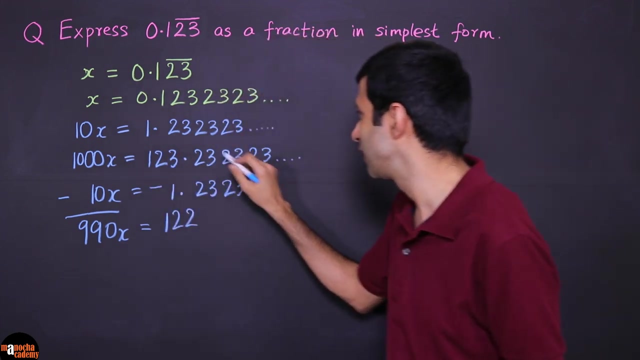 So what do we get here? This is going to be 1000 minus 10x, So that's 990x, Right, And that's going to be equal to 100x 122.. Because this? So, when we subtracted these two numbers, 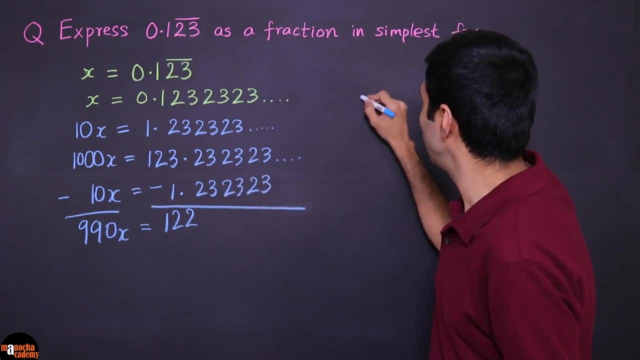 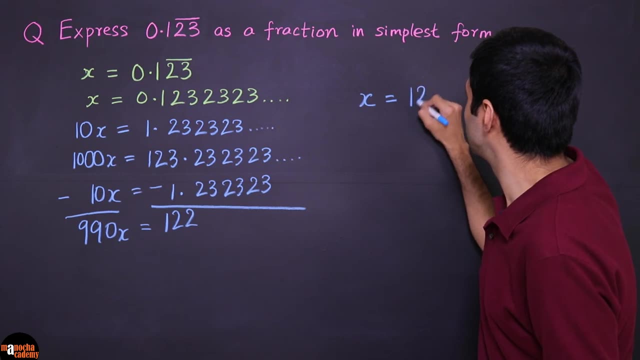 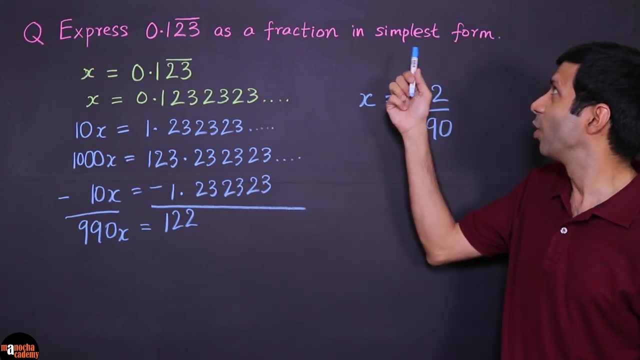 this entire part got cancelled. So what is x going to be? So x is going to work out to be 122 by 990.. So should we leave the answer like that? No, We want it in its simplest form. 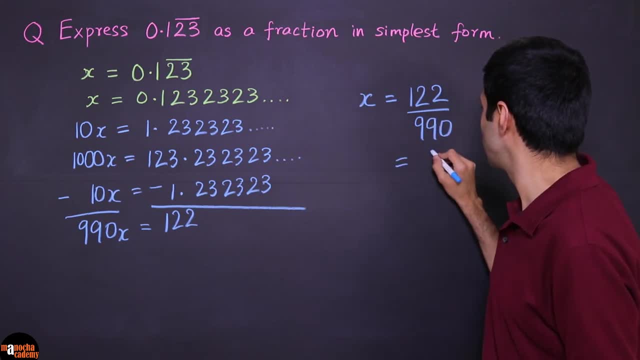 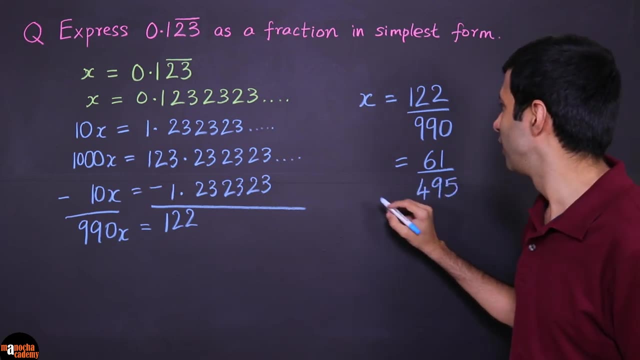 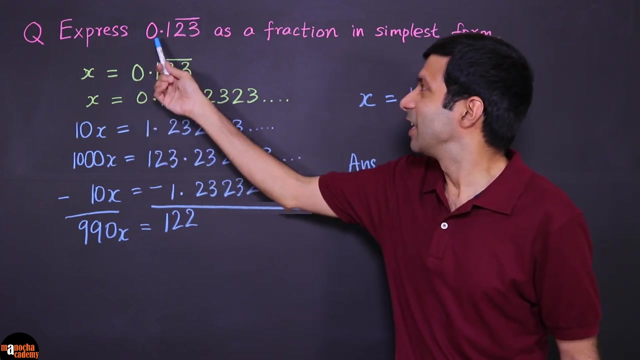 Right, So let's cancel out any factor here. So it's by 2.. Right, So it's going to be 61 by 495.. So that's our answer. Okay, That this decimal 0.123. 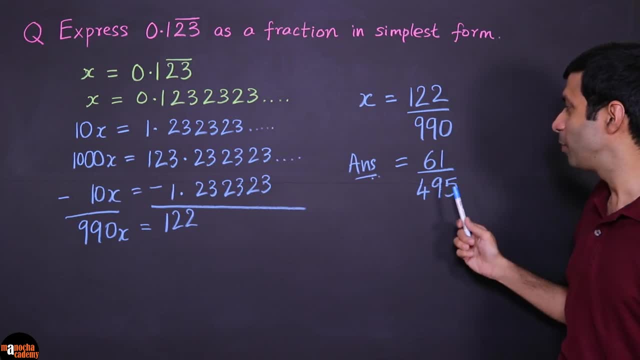 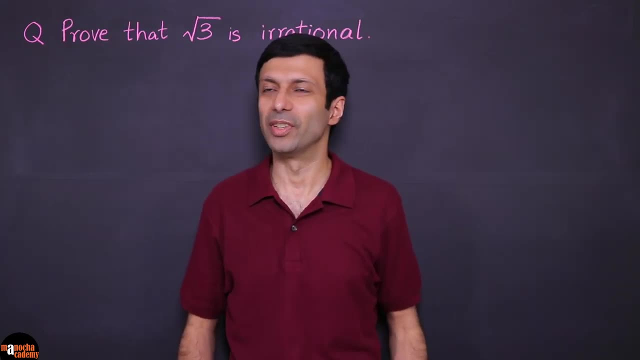 with the 23 recurring part can be written as 61 by 495.. So that's the fraction in its simplest form. Now let's take a look at the next question. Prove that root 3 is irrational. Okay, So we know that root 3. 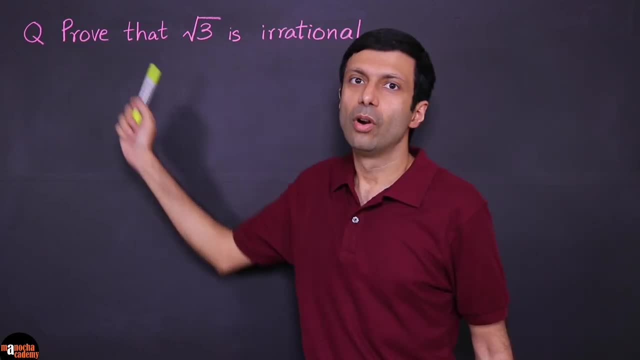 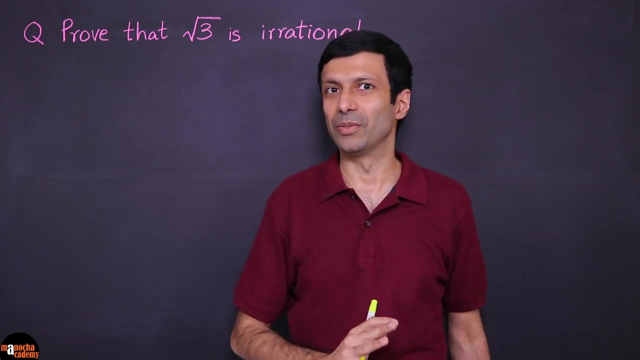 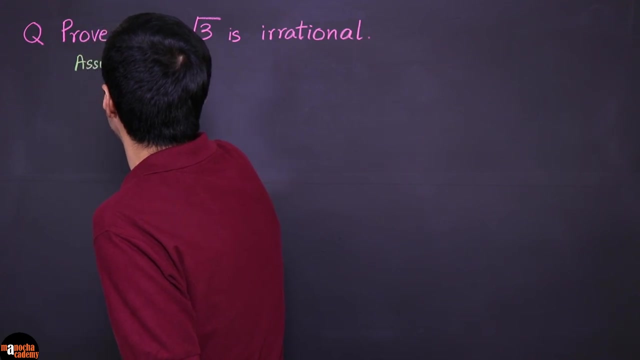 is an irrational number, But in this question we need to prove it. So what is the trick of this question? We can prove this by contradiction, So we are going to assume first. So let's assume that root 3 is. 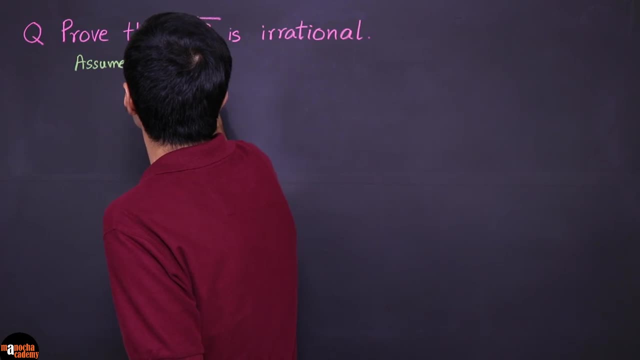 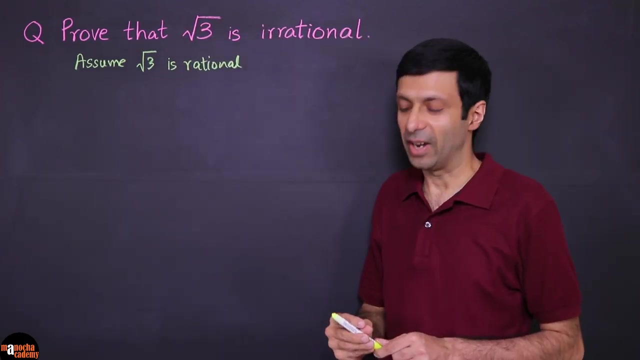 a rational number. So assume that root 3 is rational, And if we can prove this assumption is false, it will mean that root 3 is irrational. Okay, So if I assume that root 3 is a rational number, then I can write. 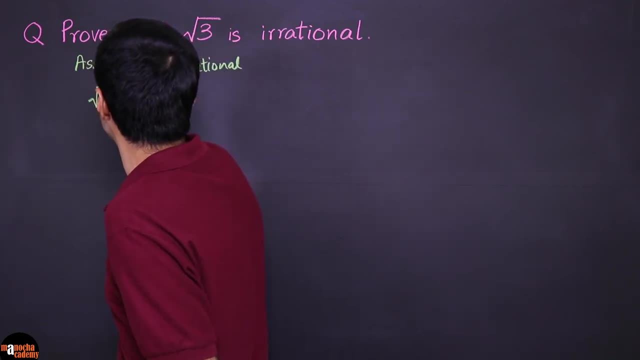 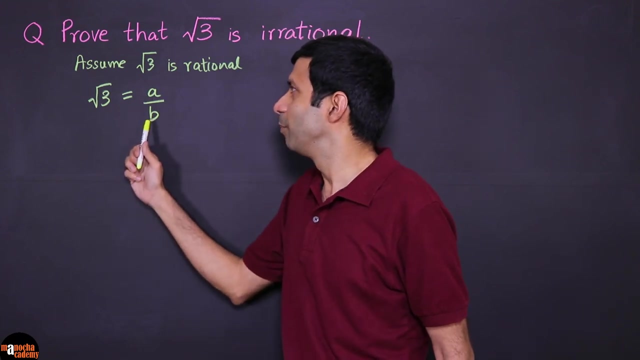 root 3 in the form of, in its simplest form, a by b. Okay, So here, a by b is the simplest form, because we are assuming it's a rational number And this means that the denominator b is not 0. And since it's 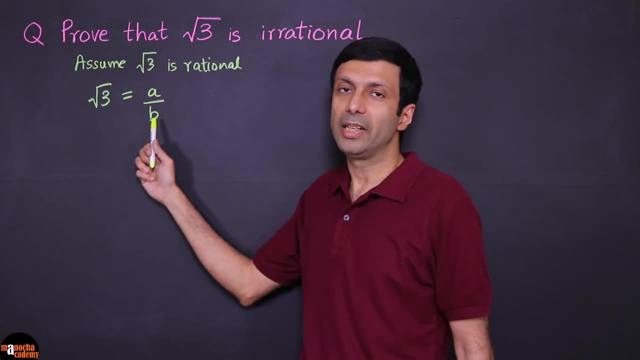 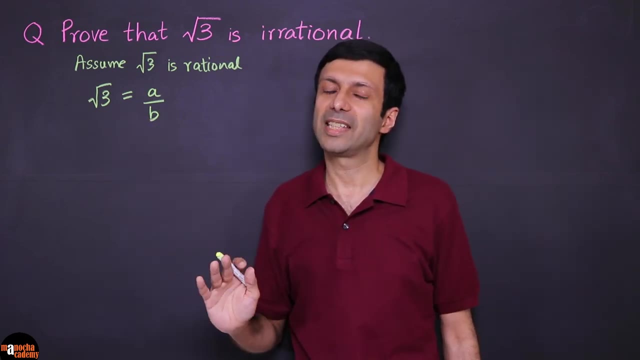 the simplest form, a and b don't have any common factor except 1.. Okay, So if I assume that root 3 is a rational number, then I can write root 3 in the form a by b. Okay, So let's. 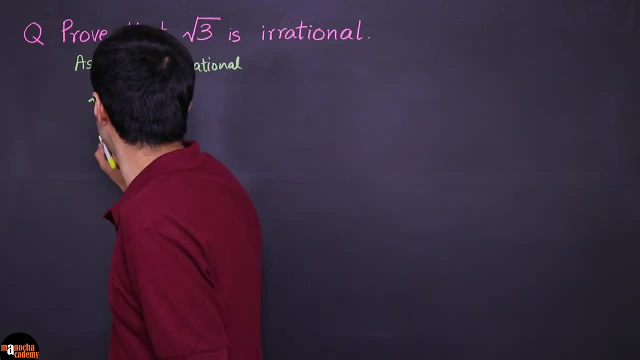 start with that. Now, the first thing you can do is let's square both sides. So in squaring both sides, we will get 3 equals a square by b square Right. And now, if we cross, multiply, we are going to get: 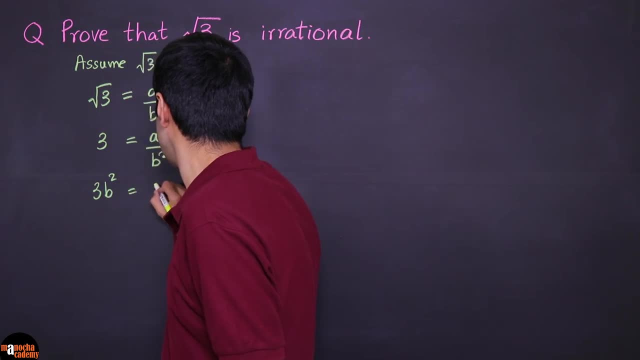 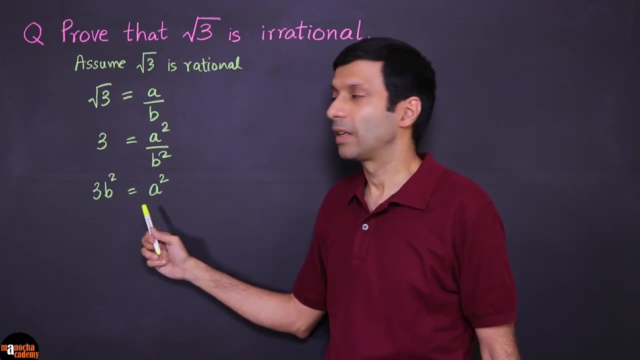 3b square equals. So I have taken the b square on this side, So we get 3b square equals a square. Now if you look at the left-hand side here, you can see that 3b square can be divided. 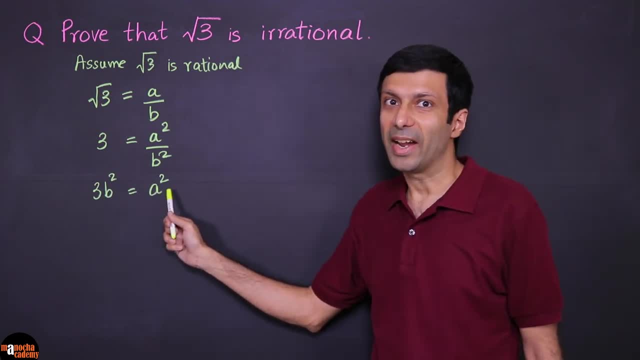 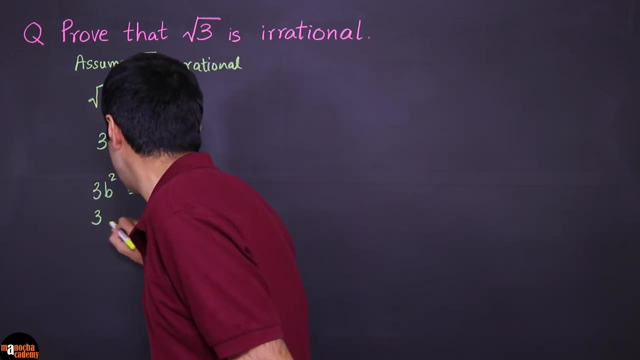 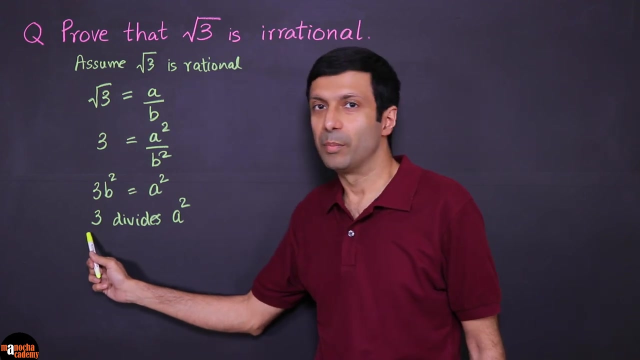 by 3.. Right, So this means that the right-hand side, a square, can also be divided by 3.. So let's write that down here: 3 divides a square. Now, since 3 is a prime number, we can also: 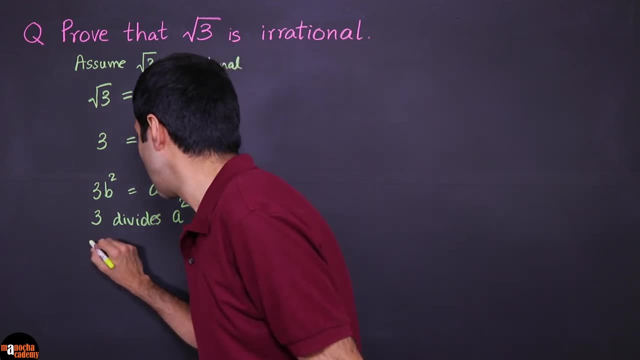 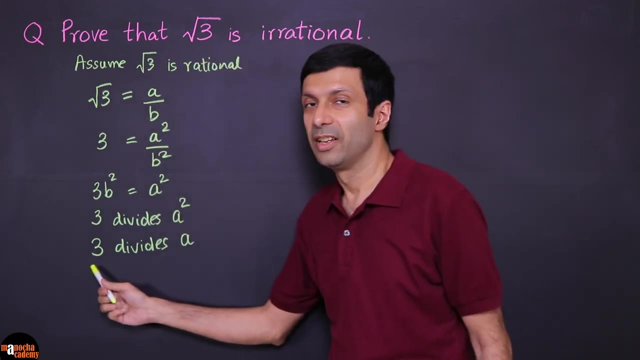 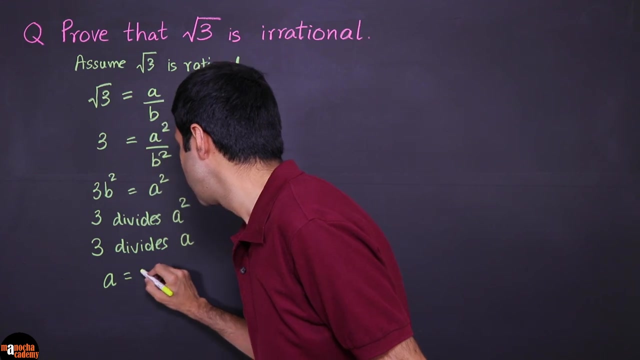 infer from here: since 3 divides a square because 3 is prime, 3 divides a Right. So this is what we can conclude from here. That means I can write a in this form: right? So we can say: 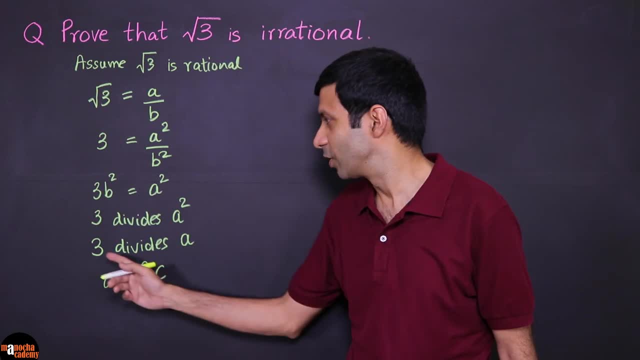 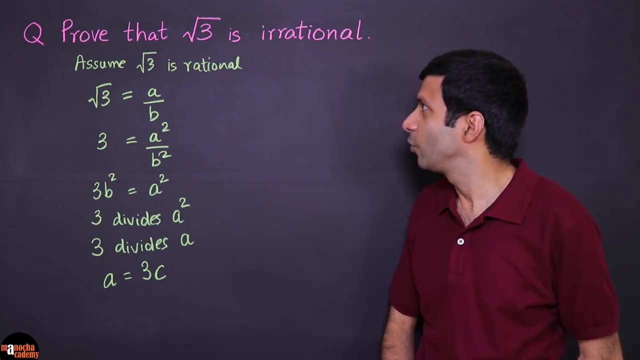 a equals 3 times a number. Let's say 3c, because 3 divides a, so a can be written as 3c. Okay, So let's use this form of substitution. We're going to substitute in this equation. 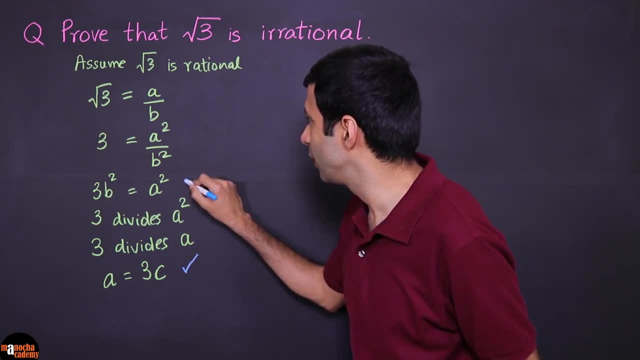 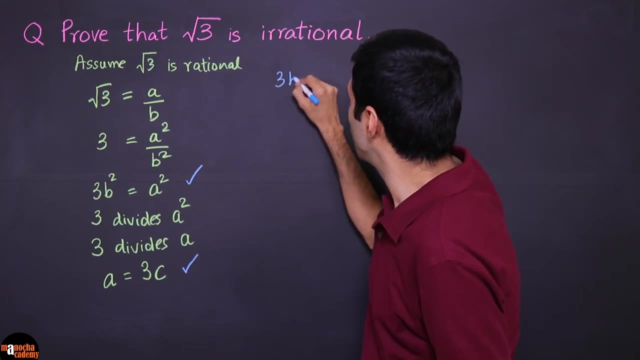 right, So I'm going to use this thing and go ahead and substitute it here. Okay, So let's write that down here. So we have got 3b squared, and instead of a I'm going to write 3c. 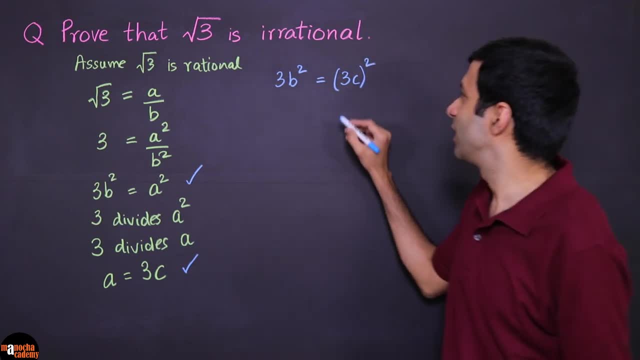 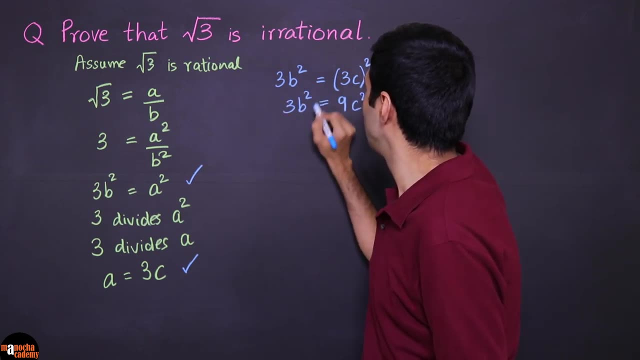 is equal to 3c whole squared Right. So let's do the square 3b squared. and, on simplification, what do we get here? b squared equals 3c squared right. So now we can apply a similar. 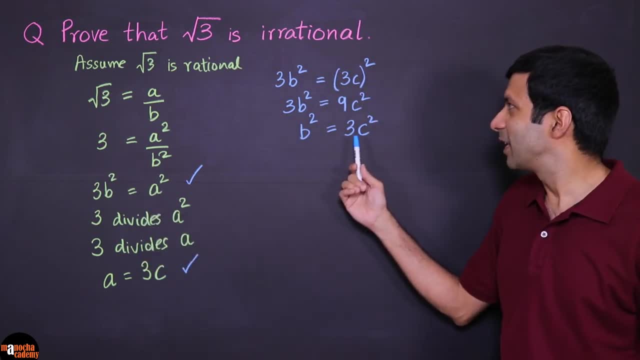 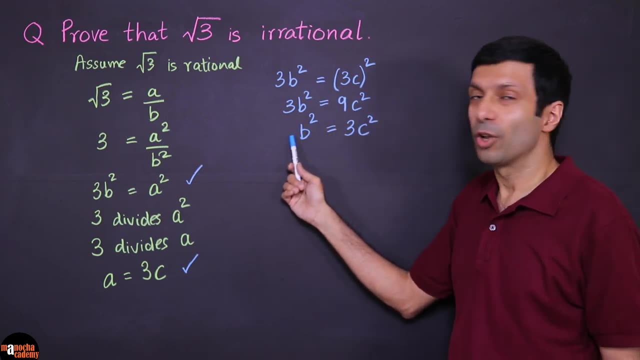 logic on, like we did here. If you look at the right-hand side here, we can say that 3 divides 3c squared right Because there's a factor of 3 here. So that means 3 will also be 3. 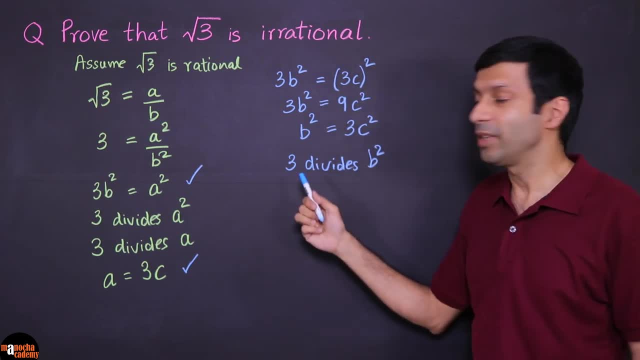 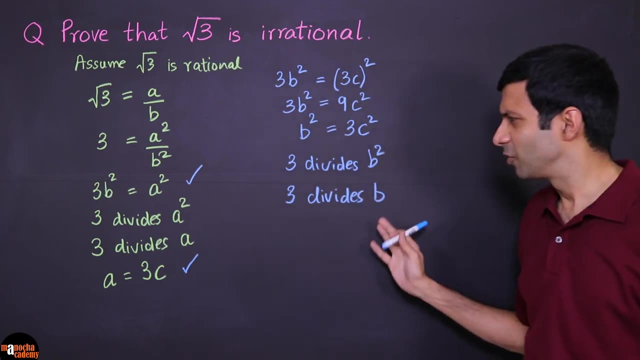 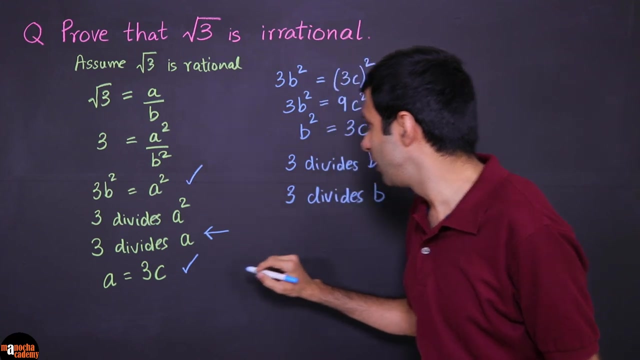 divided by b squared. And again, since 3 is a prime number, we can also say 3 divides b, correct? So it's very similar to this. So what do we have here? We have 3 divides a and 3. 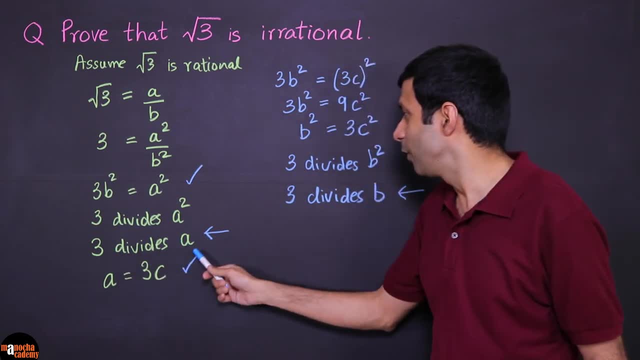 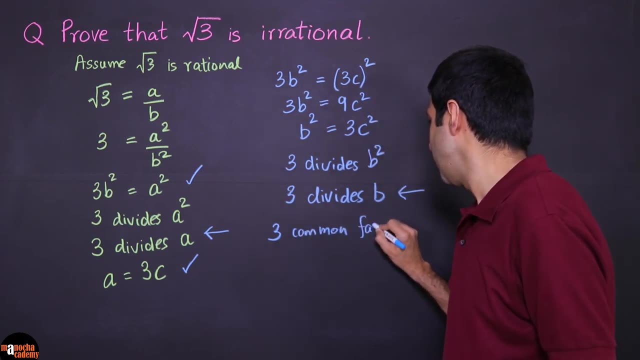 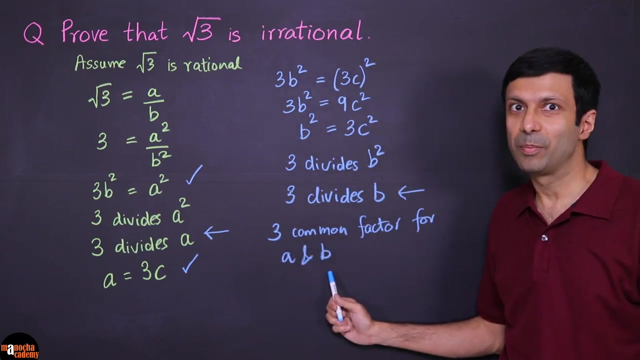 divides b. That means 3 is a common factor for. so this is a common factor for a and b. right, 3 is a common factor for a and b. Now, is that possible? No, because remember when we started here. 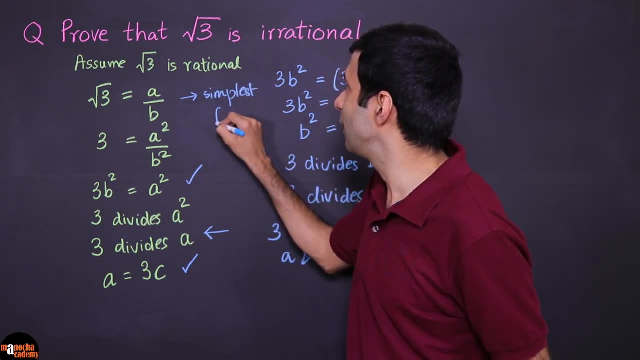 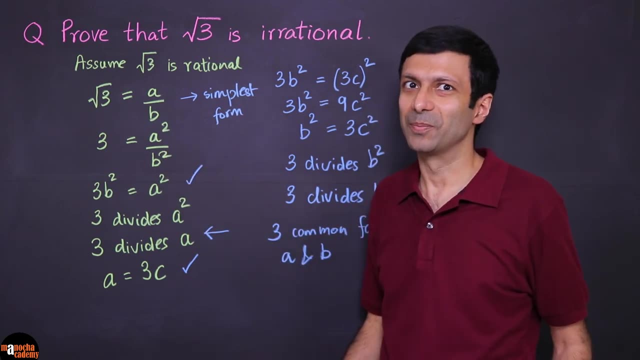 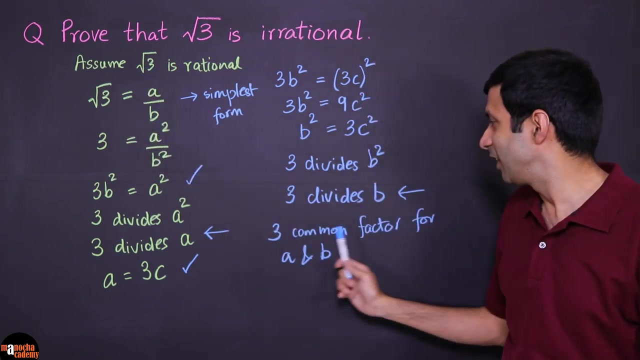 we assumed that this was the simplest form. So we assumed that we are writing root 3 in its simplest form as a by b. So this is a contradiction here, right? Because we are saying it has a common factor of 3, but 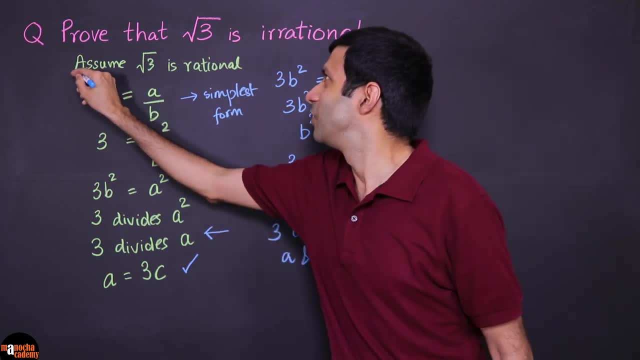 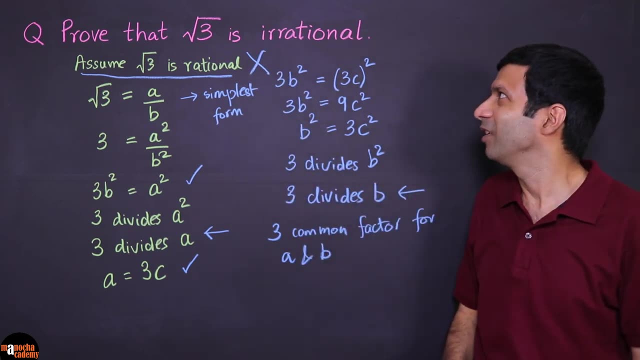 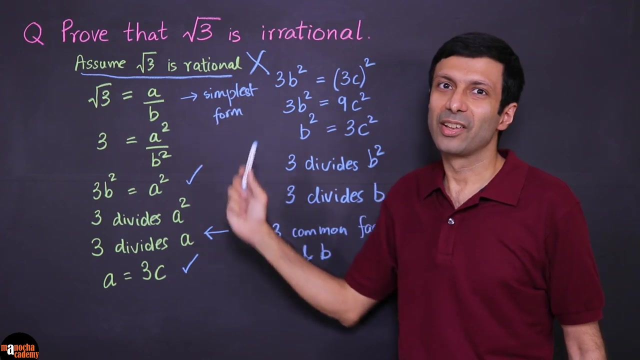 here we said that it has no common factor. So that means, because of this contradiction, our assumption that root 3 is a rational number is wrong. And since this assumption is wrong, this proves that root 3 is irrational. Now let's: 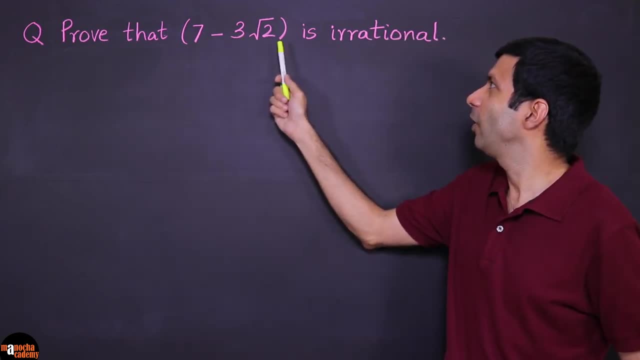 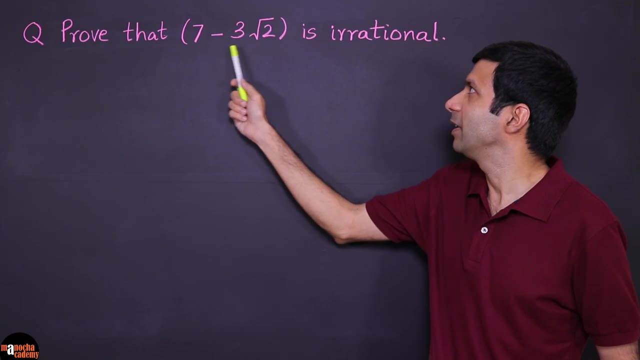 go for this question, Prove that 7 minus 3 root 2 is irrational. Okay, So let's take a look at the number that we've been given: 7 minus 3 root 2.. Okay, So one is if 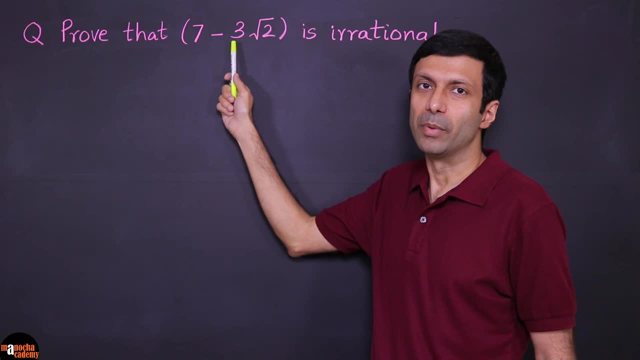 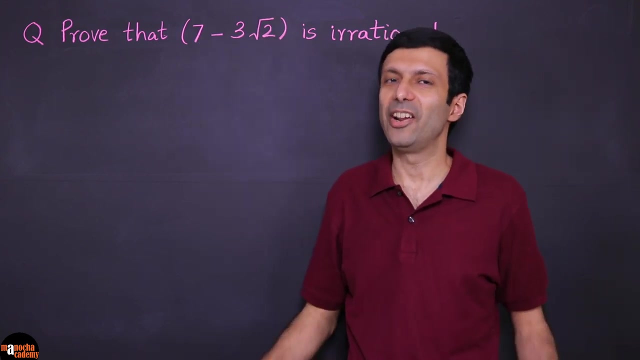 you apply common sense here, can you see that root 2 is an irrational number and 3 is a rational number, And if you add or subtract a rational and an irrational number, you're going to end up with an irrational number. So that's. 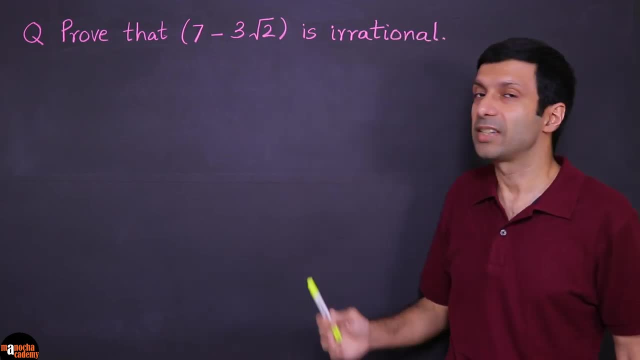 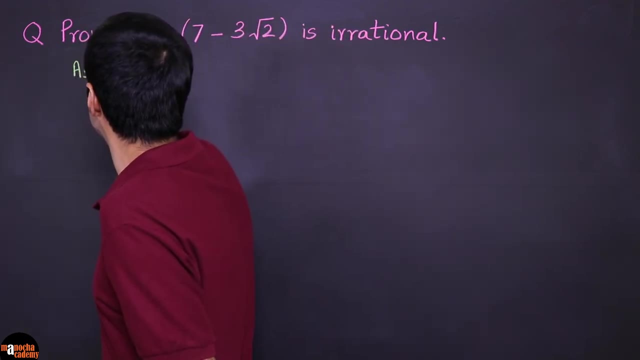 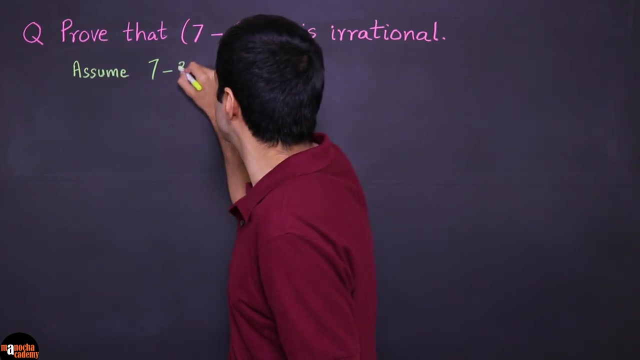 one way to explain this, But let me show you a more formal proof where we are going to start again with the contradiction technique. Okay, So again we are going to assume that. so let's say that root 2 is a rational number. 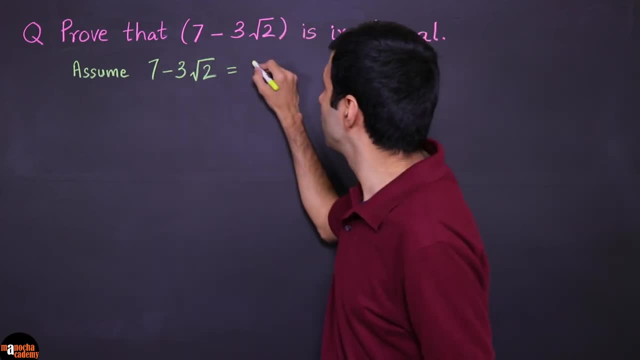 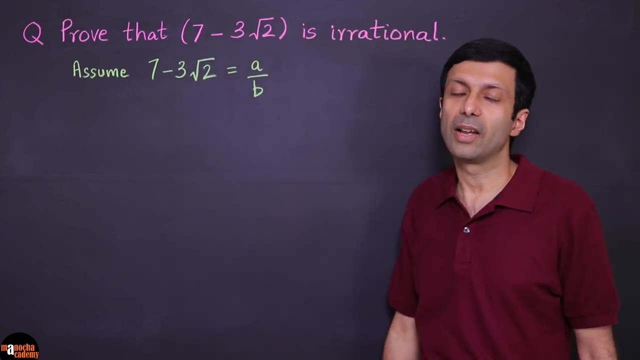 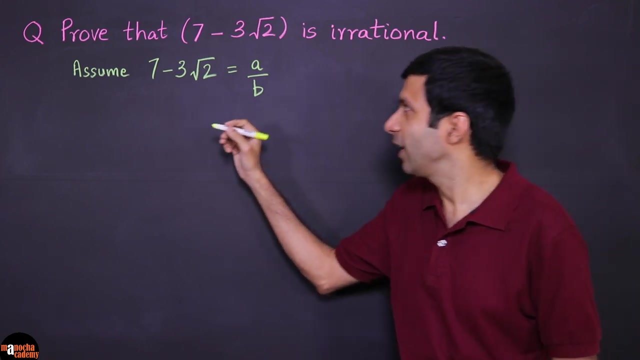 So that again can be written in the form of a by b- Let's say that's its simplest form- where b is not equal to 0 and these don't have any common factors. Okay, So let me bring this term to the. 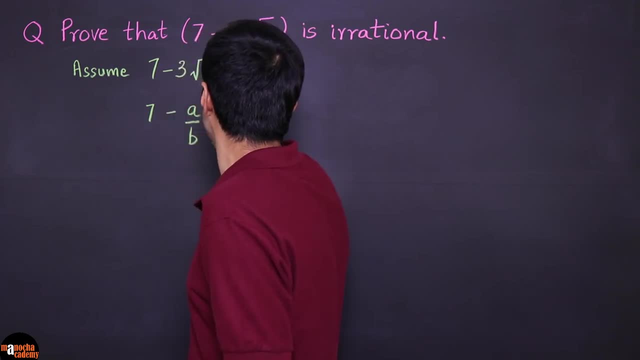 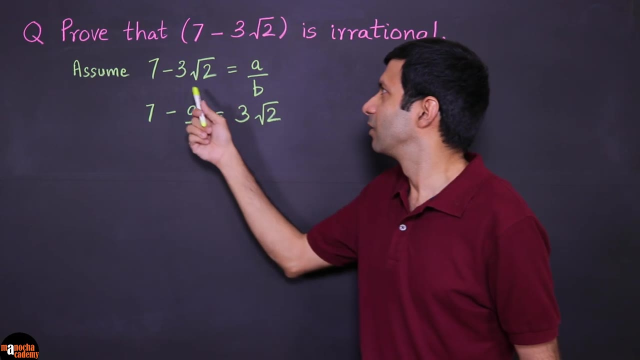 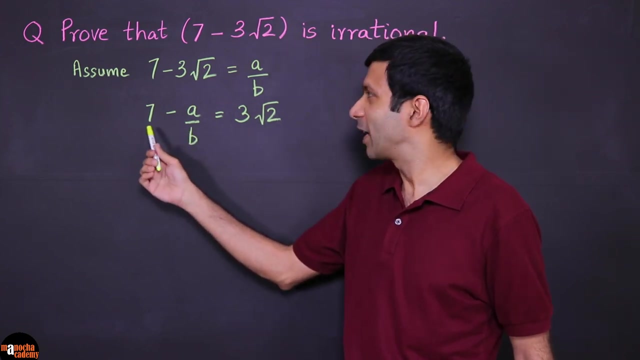 right side and this one to the left and this one to the left. Okay, So we just rearrange this equation and if you look at the left hand side here, can you see that we are subtracting two rational numbers, because 7 is. 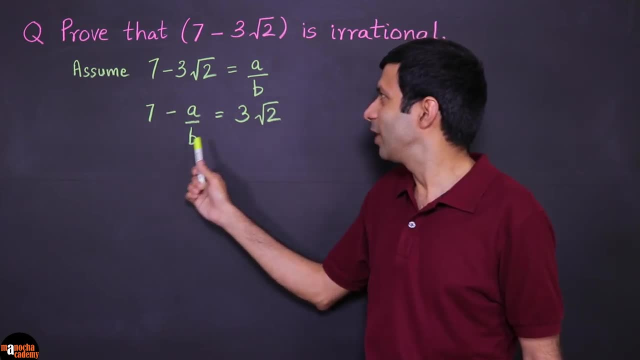 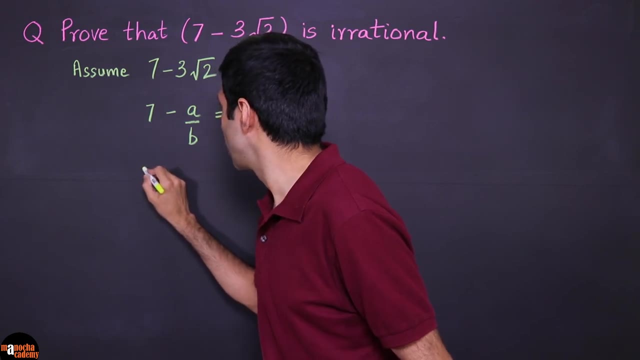 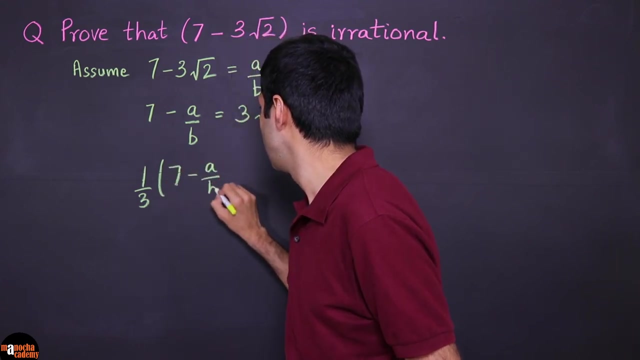 rational and a by b is rational. So the left hand side here is rational Right. And now let's take a look at where we are going to get 1 by 3 into 7. minus a by b equals root 2.. 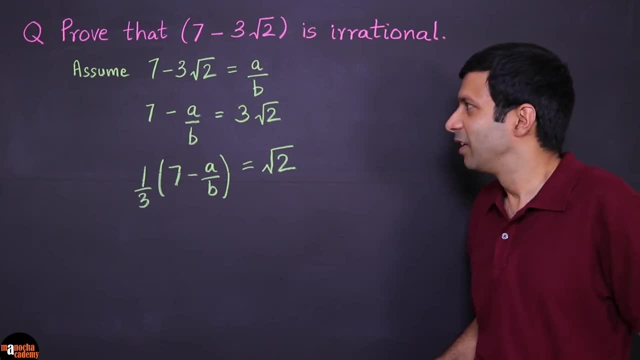 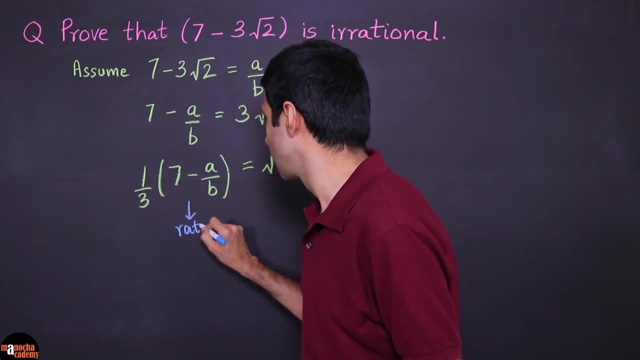 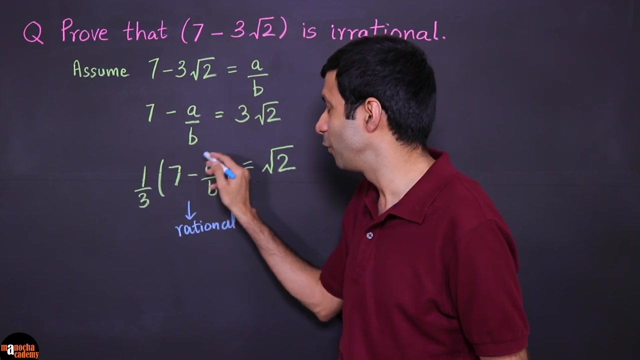 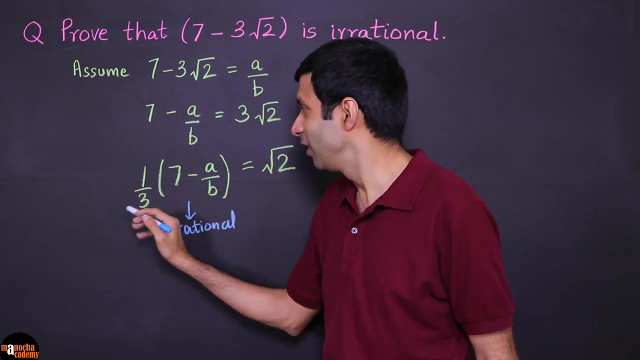 Right. So now let's take a look at this carefully. So here, as we said, 7 minus a by b is going to be a rational number, because 7 minus a by b is going to be a rational number. So if 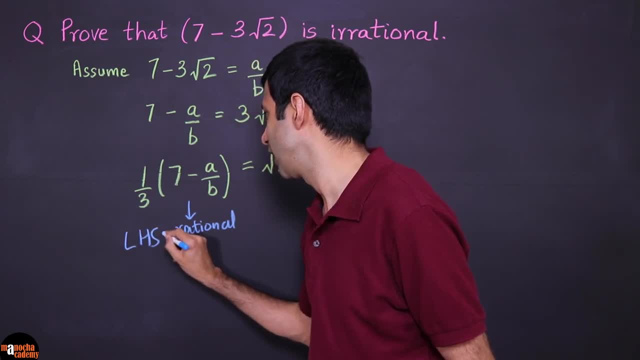 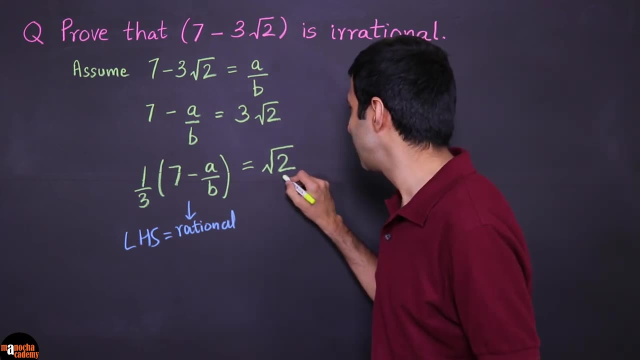 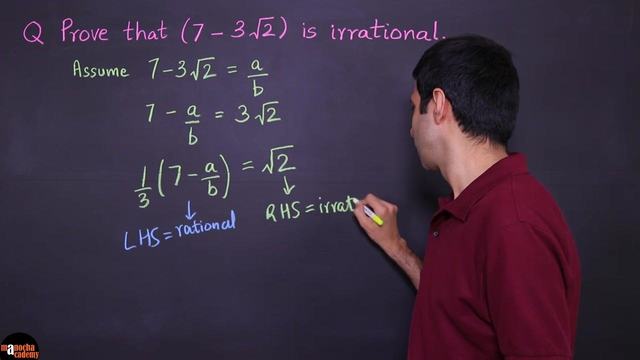 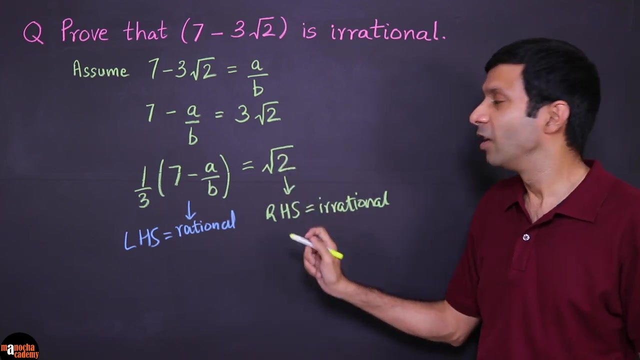 we divide this number, which is a rational number, with 3, which is again a rational number. so dividing a rational by a rational, so this entire left hand side is going to be a rational number, Right? So if we know that root, 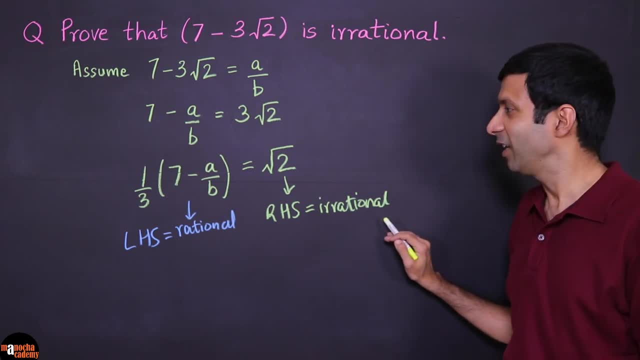 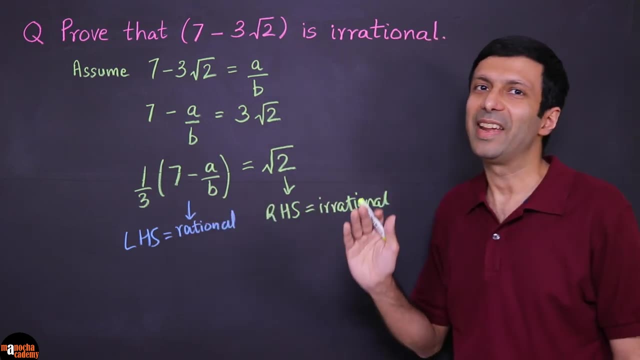 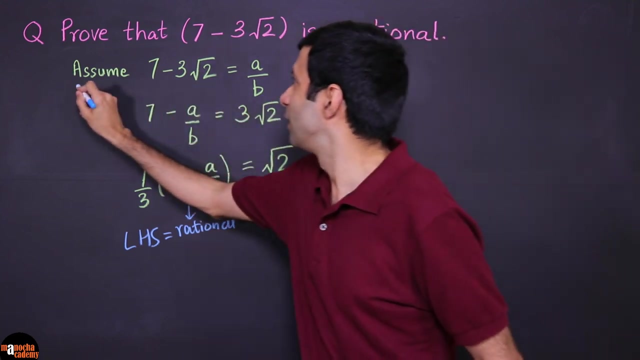 2 is a rational number. we can take it, because we know that root 2,, root 3, these are irrational numbers, Right? So can you see the contradiction that we have here? The left hand side is a rational number. 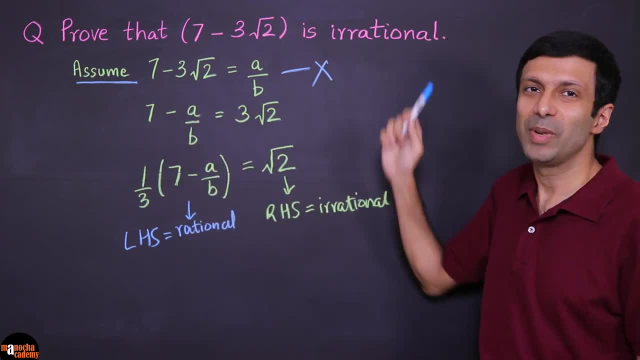 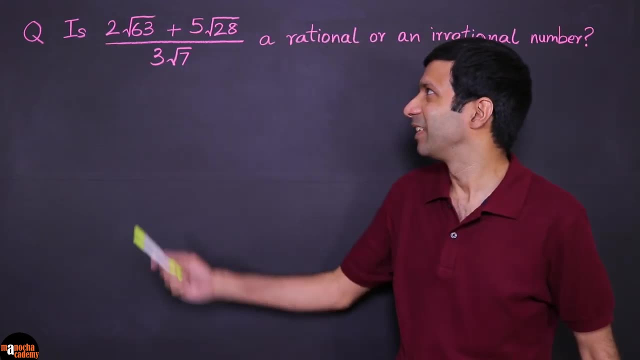 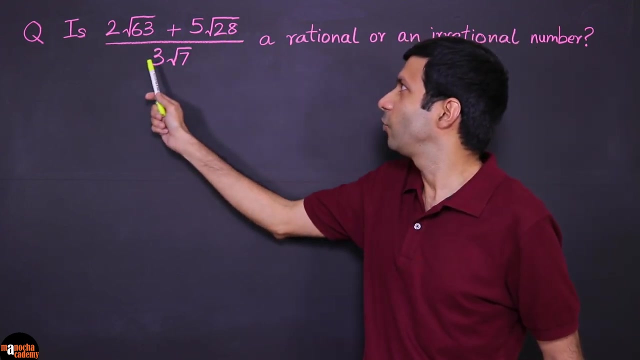 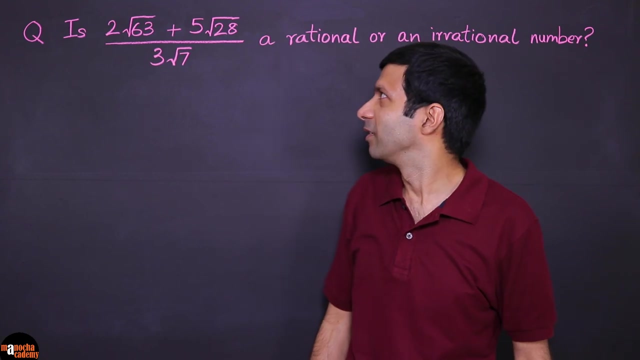 but the right hand side is an irrational number, so it must be an irrational number. So again, we proved this question using contradiction. Now let's look at this question: Is 2 root 63 plus 5 root 28, divided by 3? 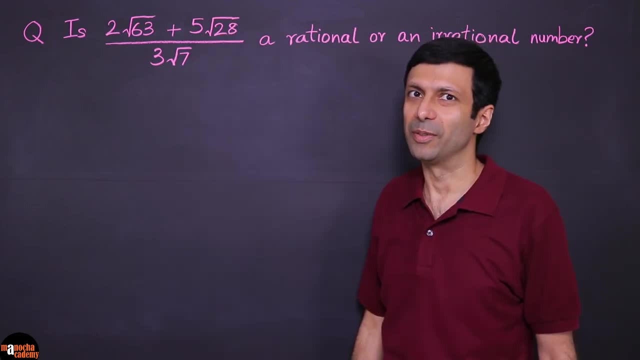 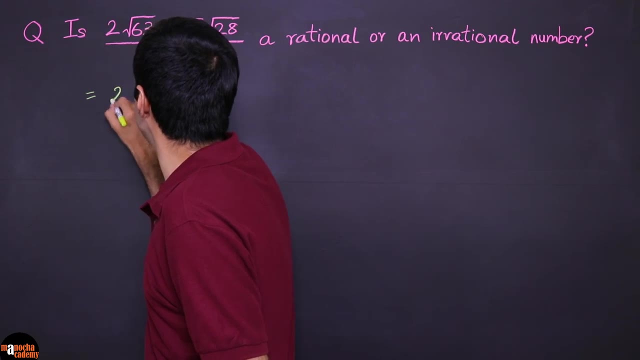 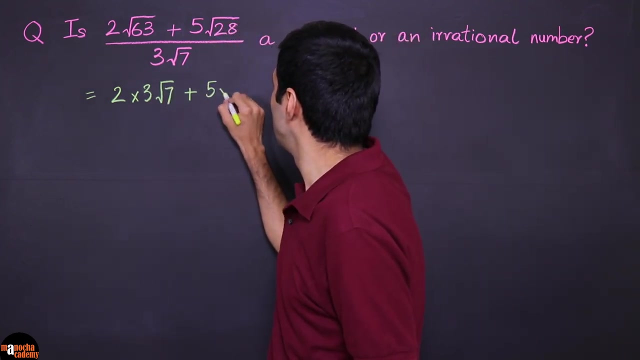 root 7?. So if you simplify this fraction that we have been given, okay, so let's go ahead and write down this as so. this number is going to be basically 2, and you know that root 63,, so that's. 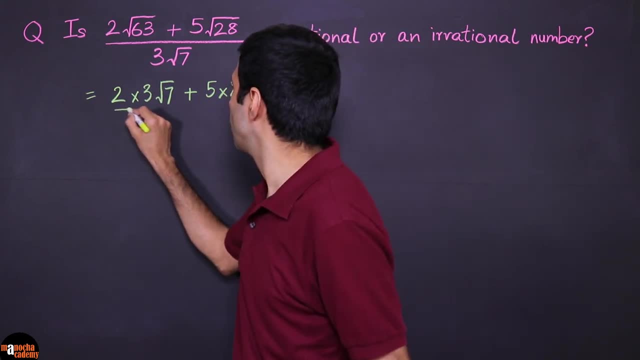 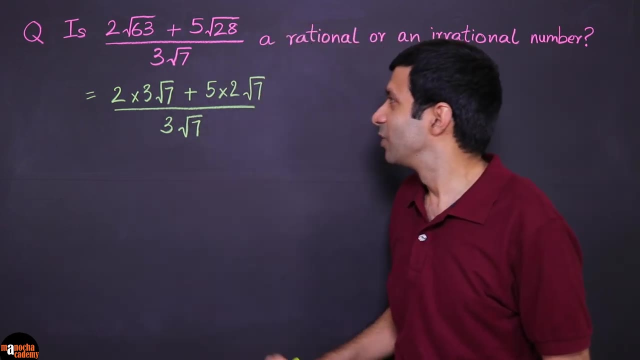 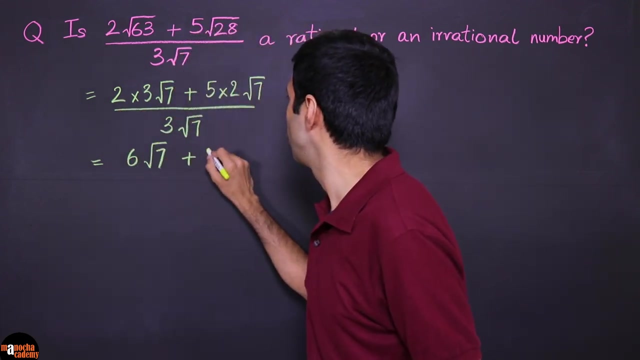 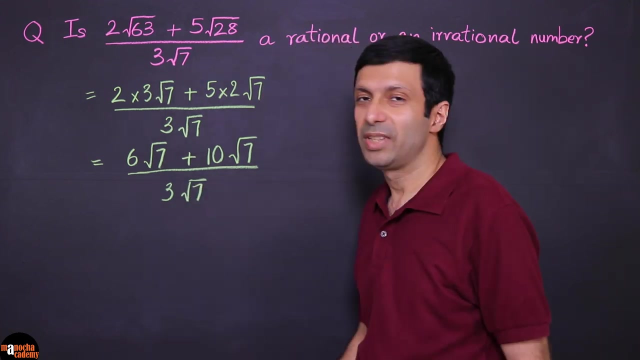 9 into 7, right, So we just write down the denominator here, because the denominator we can't simplify further: 3 root 7, okay, So now let's go ahead and write this as 3: 2's. 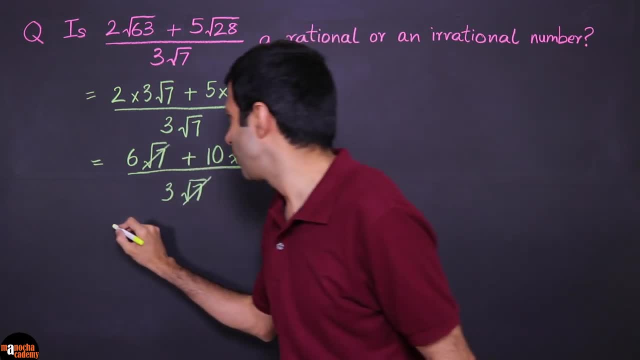 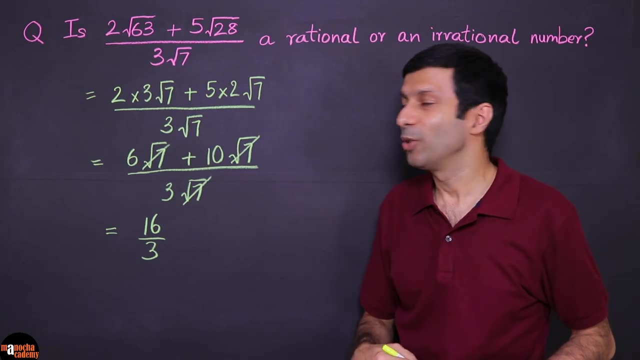 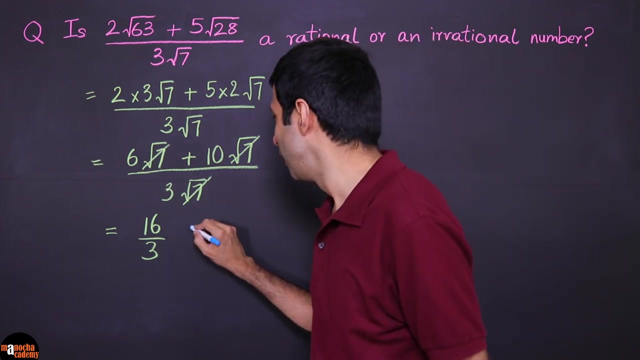 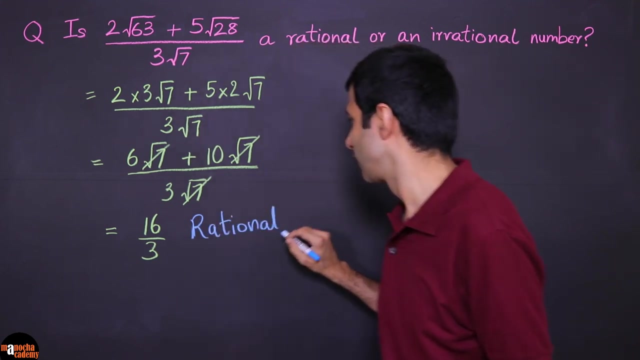 as 6 plus 10 plus 16 divided by 3.. So what do you think the number that we have? Is it rational or irrational? That's right. it's a simple p by q form, so we have a rational number.